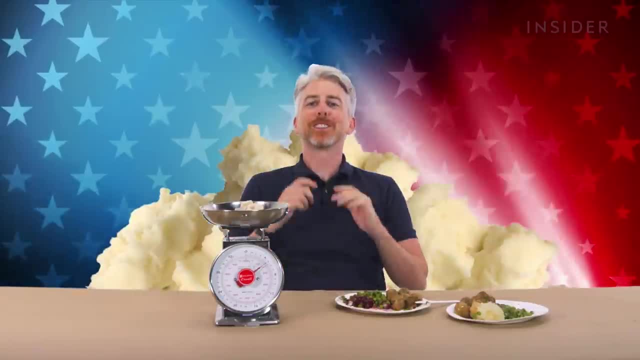 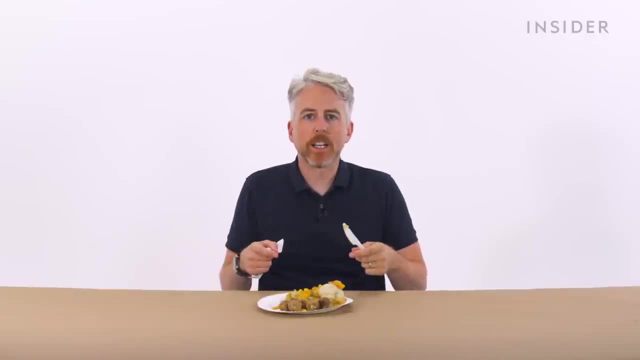 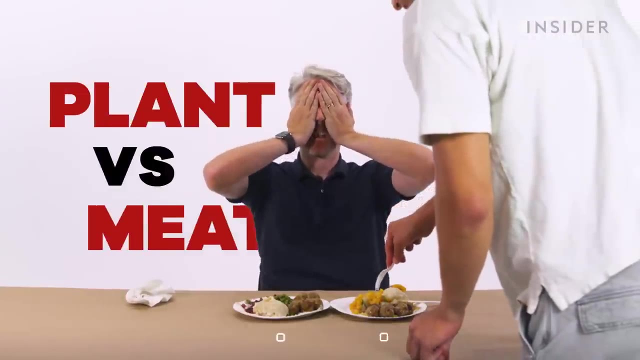 They're feeding us at our Ikea's Vegans and vegetarians: rejoice. Ikea also offers vegetarian, vegan versions of its meatballs. right here We're doing a blind taste test: plant versus meat. That's definitely plant-based. What's the next one? 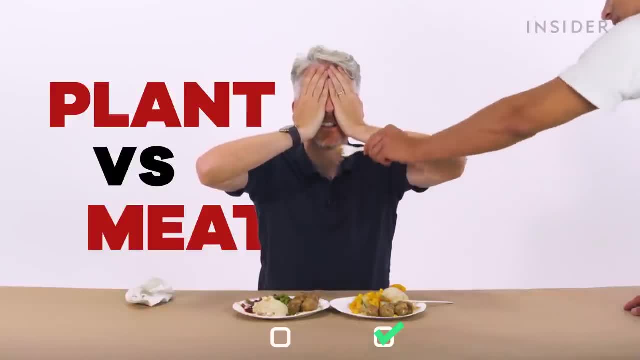 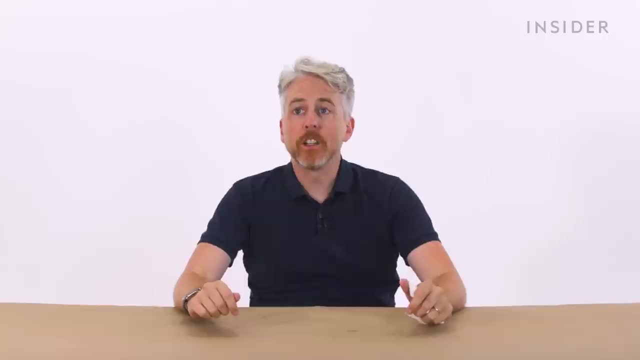 Oh, was that wrong? Wait, okay, give me the other one. Okay, this is the other one. Yeah, that's meat, Not even close. Not even close. Thank you, Peter. Neither were bad, and if I was a vegetarian or vegan? 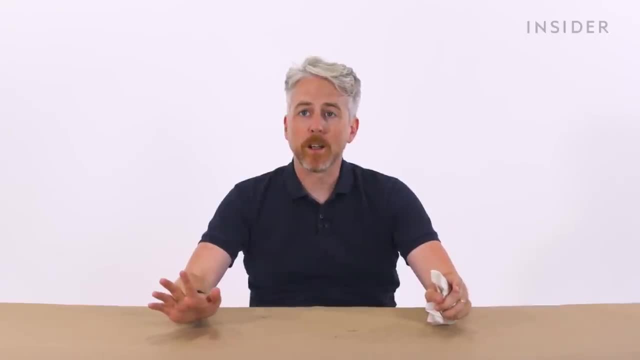 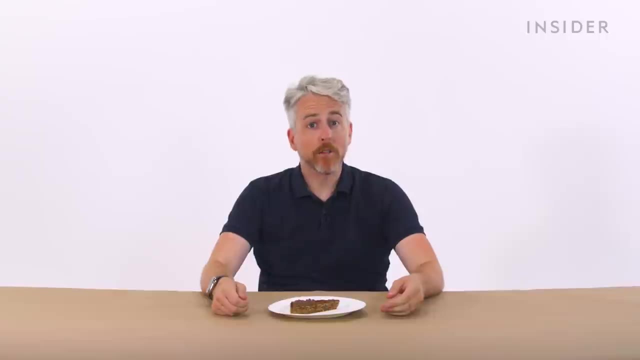 I would be perfectly happy with those. plant-based Tasted perfectly fine, but the difference is noticeable. We share a couple of dessert options with the US, notably the dime cake. Over here we call that the caramel almond cake. Let's weigh a slice. 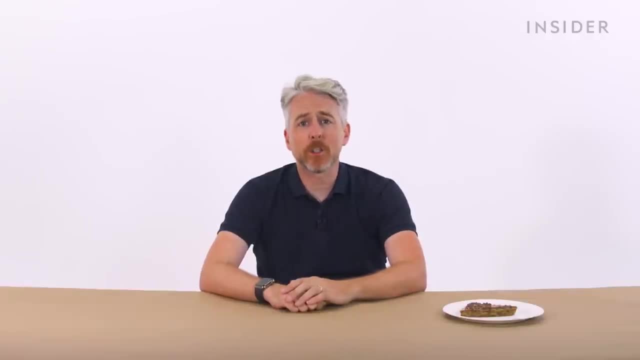 Another dessert option we share with the UK is a soft-serve ice cream, which you get in vanilla or strawberry. Okay, first of all, the gentleman who worked there was adamant that it's actually frozen yogurt. I don't know if that's true or not. 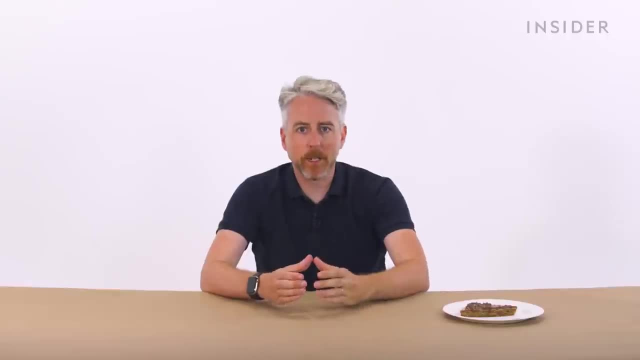 Regardless, they didn't have to-go cups like Harry was able to get, so all they would give us is like the small cup where it's kind of poking out like it's ready to eat. It is 97 degrees in Los Angeles today. 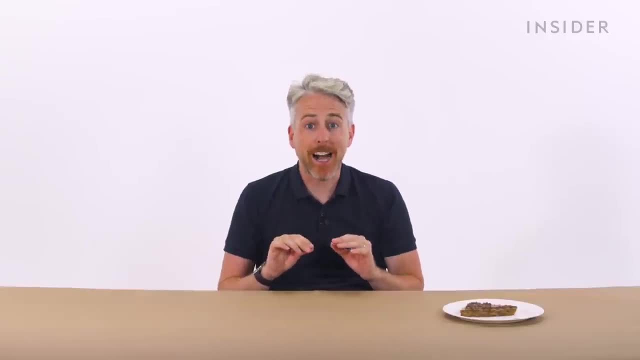 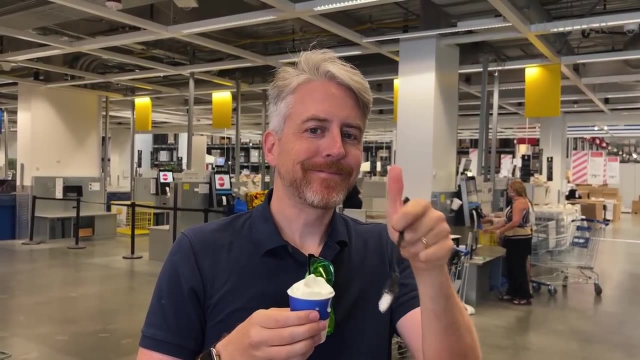 There's absolutely no way that was making it from Ikea to the car, let alone the studio. So here's footage of me enjoying it in the lobby of Ikea. So I'm sorry I didn't bring the scale. I don't know how much it weighs. 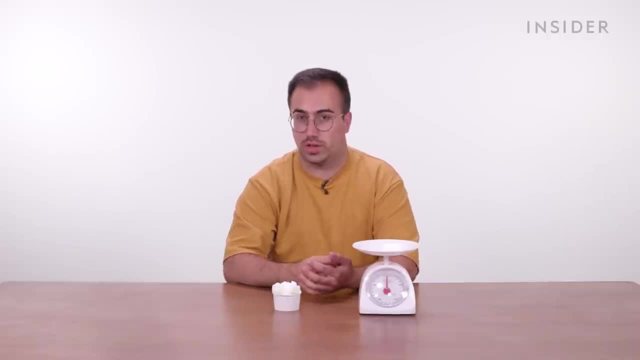 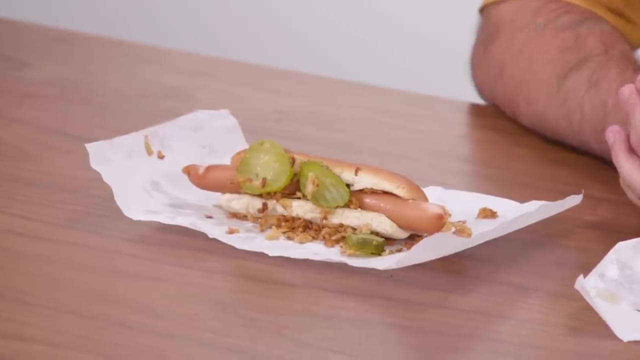 We have soft-serve ice cream in the UK too, either as vanilla or vanilla with chocolate sauce. Impressively, they've given us exactly 100 grams of soft-serve ice cream. Ikea is also known for its hot dogs In the UK. you can get either a classic hot dog 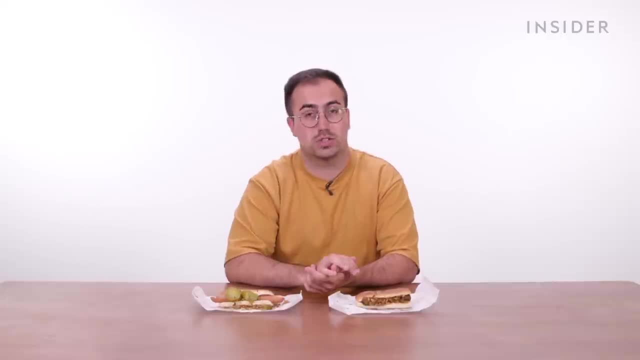 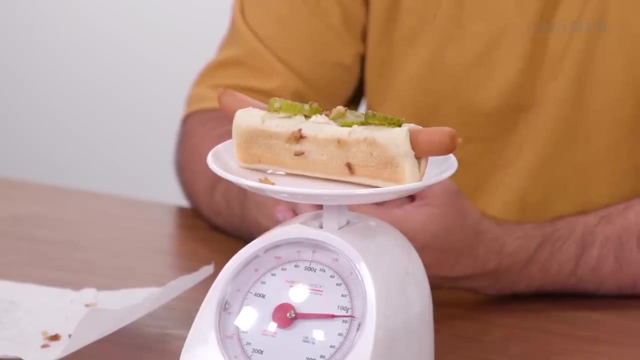 or a veggie hot dog from the bistro stand. We're gonna measure and weigh the classic hot dog. to compare with the US, The hot dog in the UK is seven inches in length and with the toppings of pickles and onions it weighs 114 grams. Hot dog. Our hot dog is 5.5.. 5.25 inches long And our hot dog weighs 75 grams. Here are all the menu items from a UK Ikea that you won't find in the US. Here's all the food you'll find in a US Ikea. 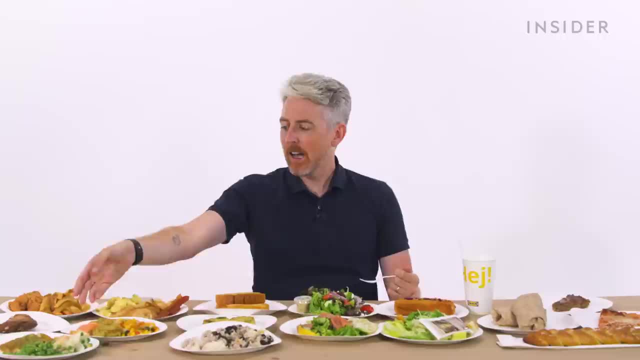 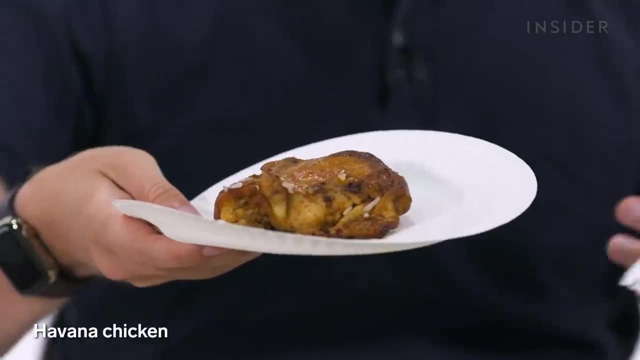 you won't find in the UK. Starting out down here, hot entrees. This single piece of chicken is the Havana chicken. Now it doesn't come alone. It comes with plantains, rice and beans, which we will see in a little bit. 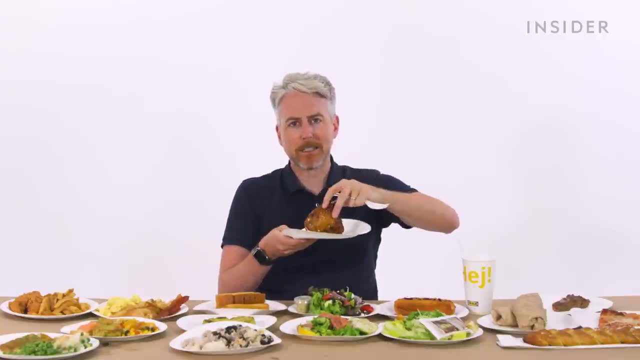 But just isolated. the chicken has been sitting for a minute. sorry Havana chicken. I wonder what makes it so, Havana? Yeah, I'm definitely getting some spices in here. Very flavorful, Not just like a standard piece of chicken, It's actually really good. 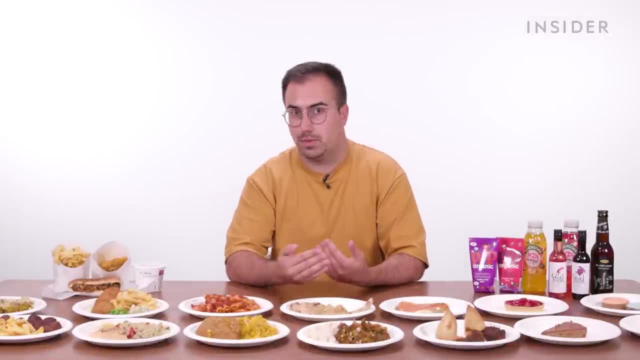 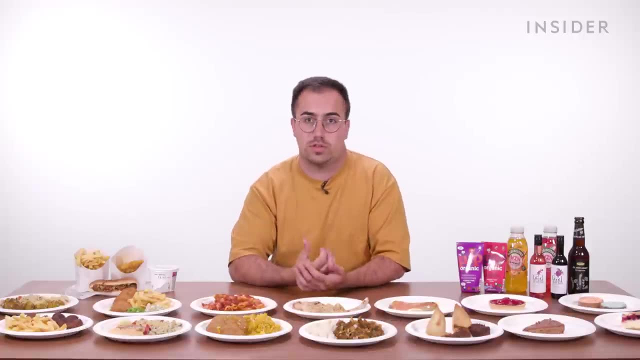 We'll start down this end with some main courses. We have two different non-meat meatball options in the UK. Firstly, we have the veggie balls. These are meatballs which are formed of ground up vegetables and they're also served with a vegetable couscous as well. 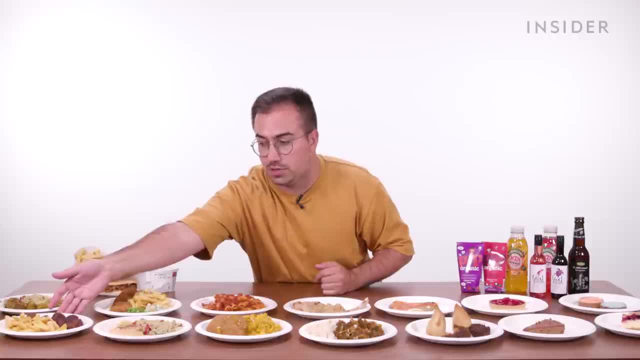 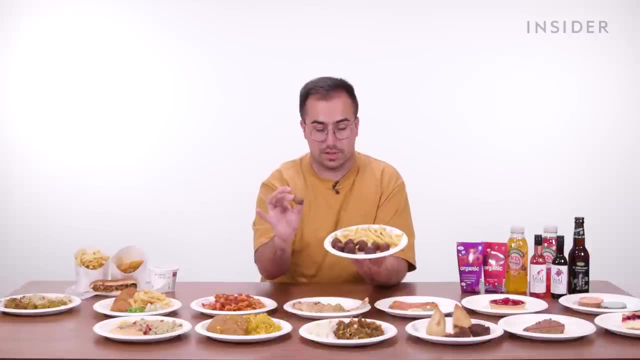 But for vegetarians who prefer something a bit more reminiscent of meat, they also have plant balls. Now, I'm kind of intrigued by these because they look really good. These are a fake meat version of Ikea's classic meatballs- Now compared to a classic meatball. 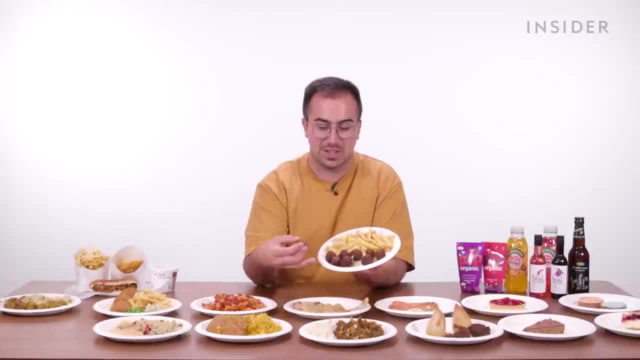 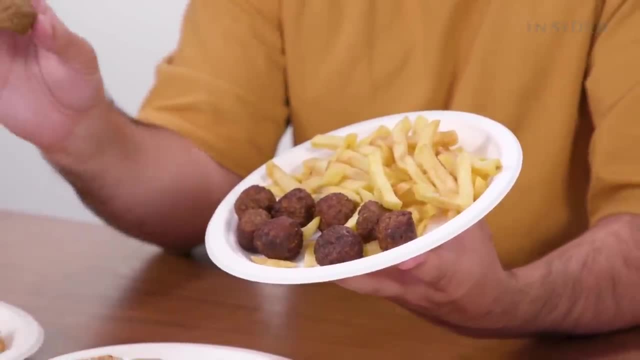 they're actually like almost more visually appealing I would say. They're a nice dark golden brown color. They look like they've been cooked in a similar way, maybe even kind of like fried or cooked, but longer than you would expect from these. 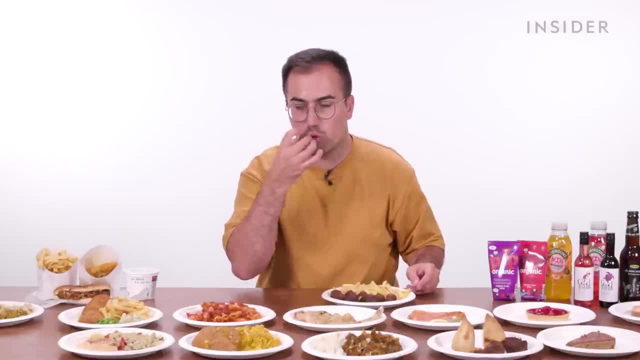 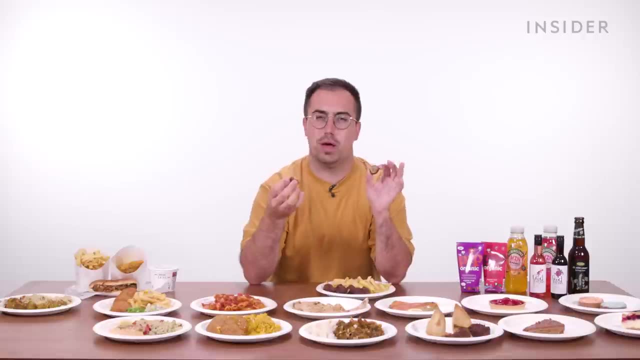 Let's do a very quick taste test. Classic meatball: We all know and love it. These things are delicious. And then one of the plant balls- I will say the plant-based one- doesn't have that distinct Ikea meatball taste to it. 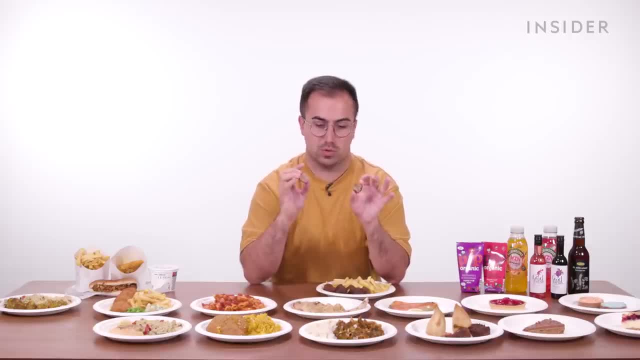 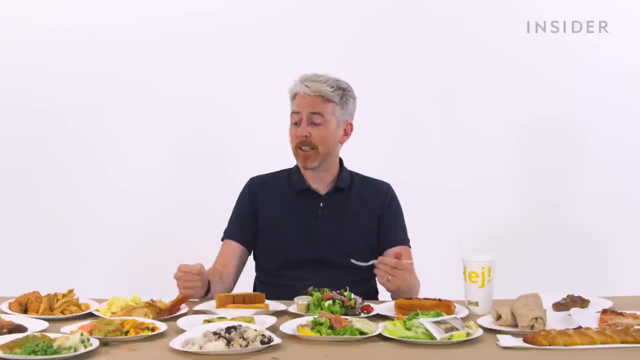 That said, still pretty tasty, I think. texture-wise it's like almost identical to the classic meatball. You can also get a salmon filet with pea pesto, vegetable medallions and a corn medley, which you can see right here. 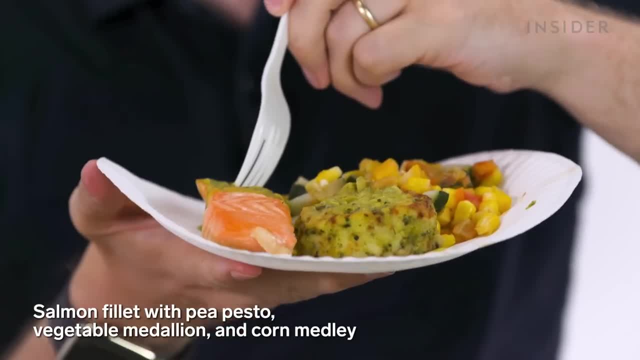 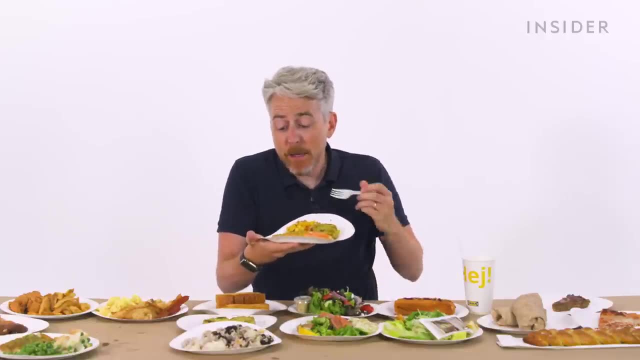 I mean salmon's. okay, I guess This isn't. it's been sitting for a while. If you like salmon- sure I don't know you- go to Ikea. you can get salmon. Pesto's interesting though. 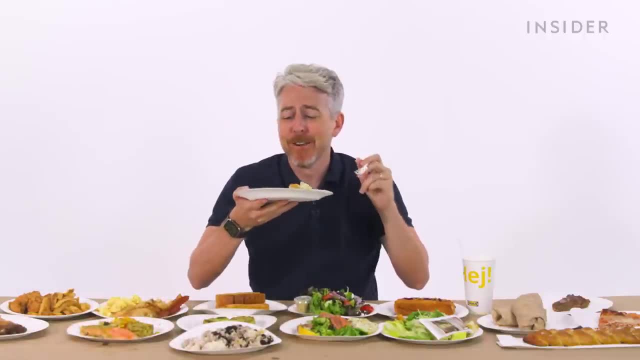 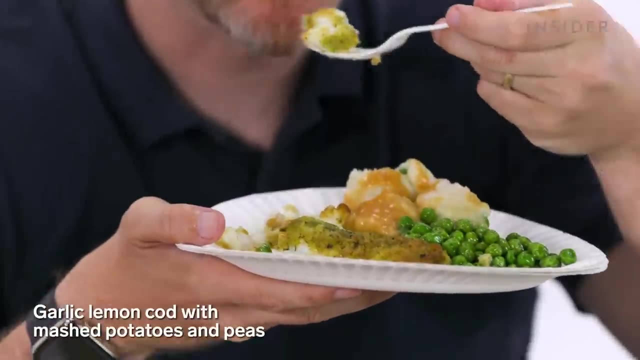 Still in the mood for fish before you go furniture shopping. You can also get the garlic lemon cod with, of course, mashed potatoes and peas. Actually, that's a pretty good piece of fish. You actually really like that. Okay, I stand corrected. 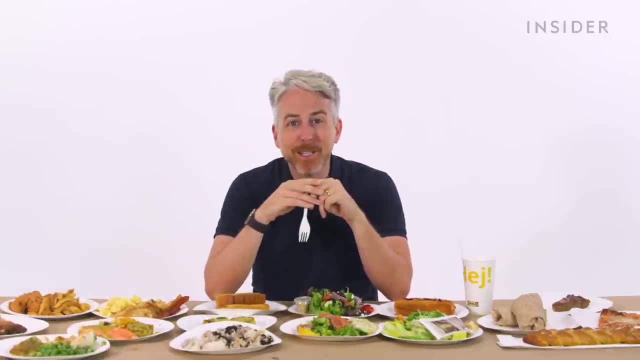 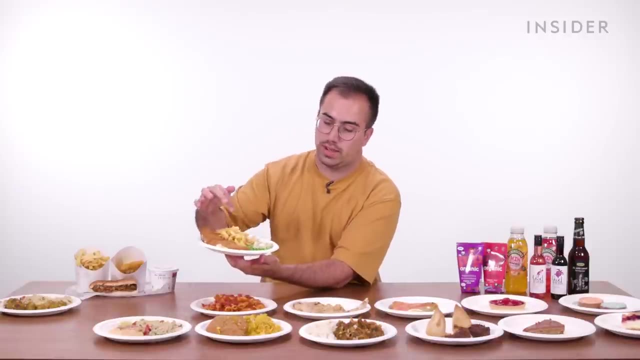 I was dissing the fish. That actually is pretty good. We have a British classic dish and that's fish and chips. Now the fish they serve at Ikea in the UK is pollock. It comes with chips, peas and some tartar sauce. 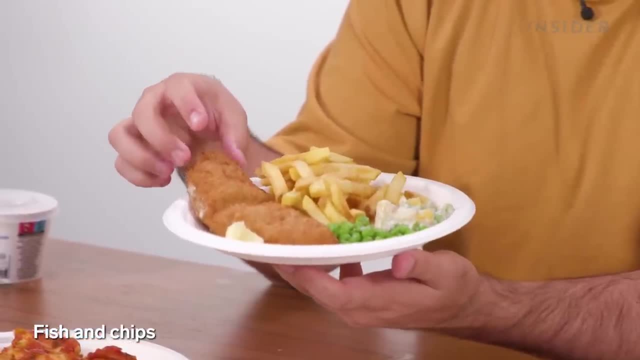 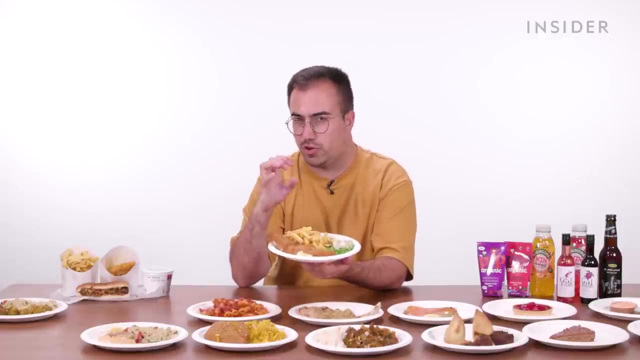 Now, unlike fish and chips that you might find from a classic chippy in the UK, they've actually breaded their fish rather than battered and then fried it. I generally prefer the battered fish texture. I like the kind of crispy crunch on the outside. 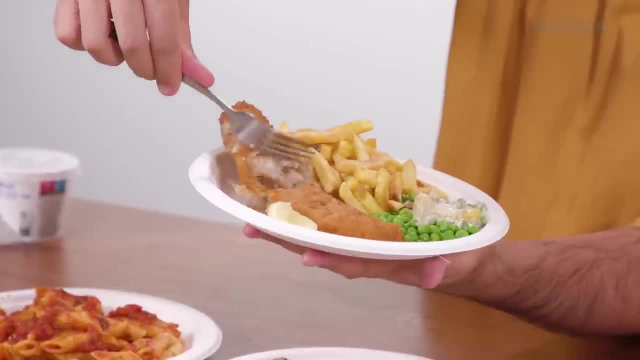 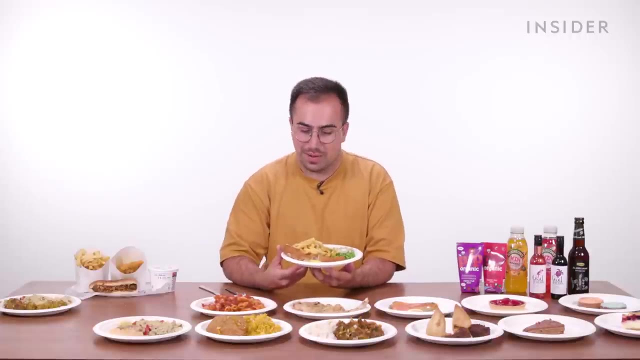 that you get from batter. I'm gonna have a little little try of this. It's very weird tasting things on Food Wars using a knife and fork. I don't like it. I respect that. they have attempted to localize their menu to the UK market. 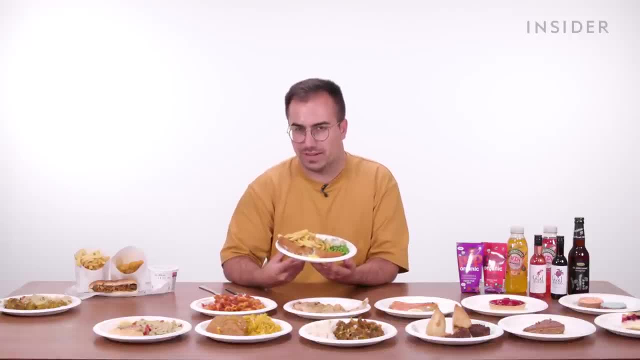 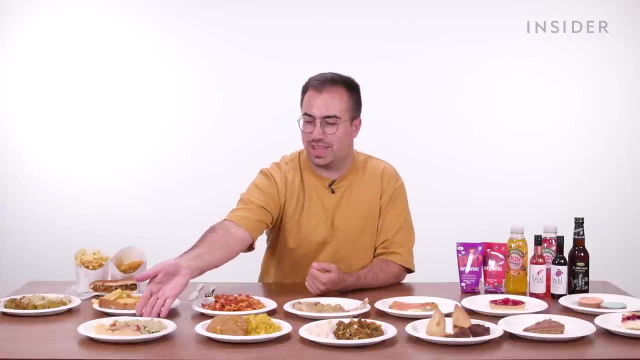 but maybe add a bit more thought into your R&D there. If you wanna see what proper fish and chips looks like, go and check out our Food Tours. Best Fish and Chips in London- video. Next up we have another fish option. It's a salmon fillet. 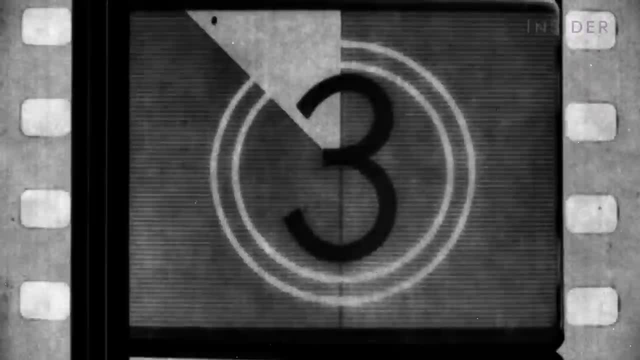 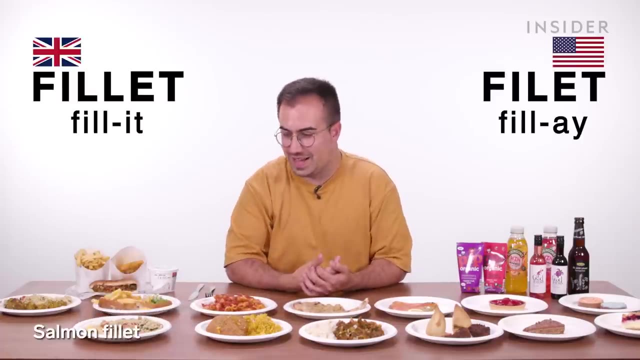 Fillet. Come on Next up. we have another fish option. It's a salmon fillet. In the UK we generally lean more towards fillet as the wording and also we spell it slightly differently. Often we spell it with two Ls. 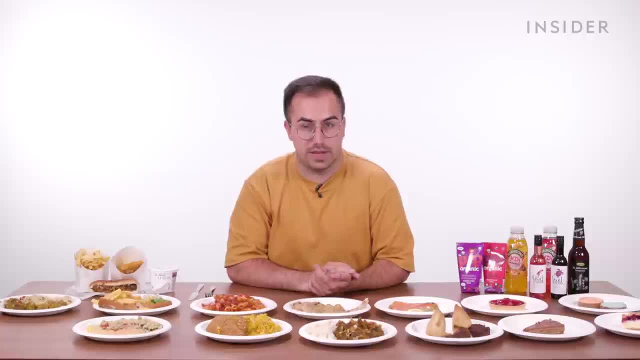 whereas I believe in the US it tends to be spelled with one. I think you can get a salmon fillet in the US. However, like we say, we pronounce ours slightly differently, And also in the UK we call it the veggie couscous. 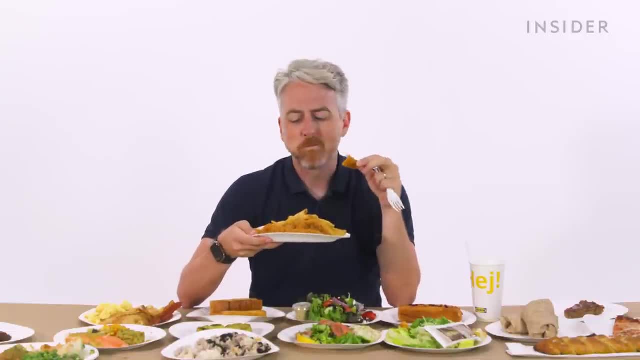 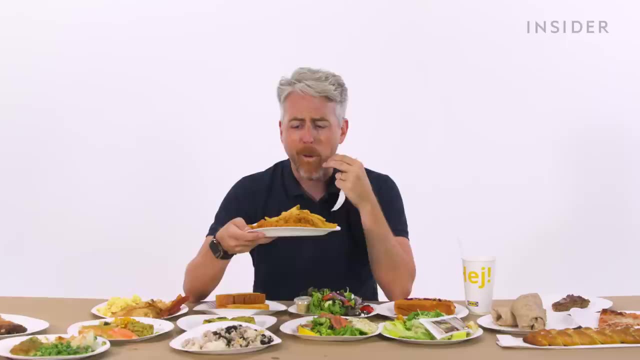 Chicken tenders, Let me go. Oh, the fries and broccoli. Mm Wait, These tenders are actually very good, Like the breading. They're really breaded Cheese and fries, hearty. IKEA also has a few things on the menu. 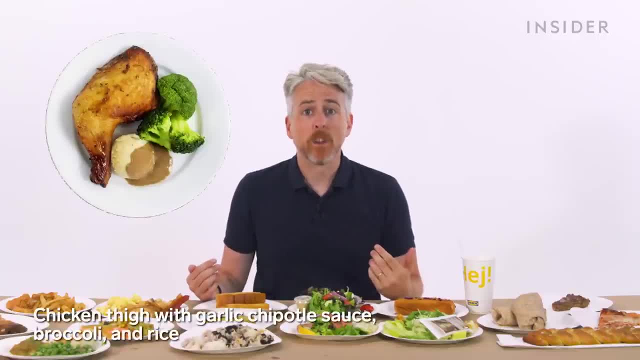 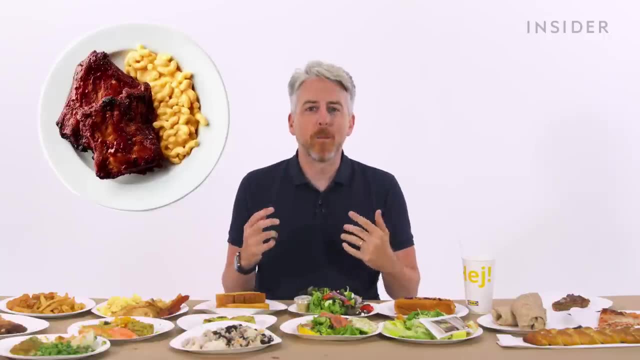 that were not available at the one we went to: A chicken thigh with garlic, chipotle sauce, broccoli and rice. It sounds actually pretty good. Lingonberry barbecue ribs with mac and cheese- Ah, I was so mad. And a plant-based burger with fries. 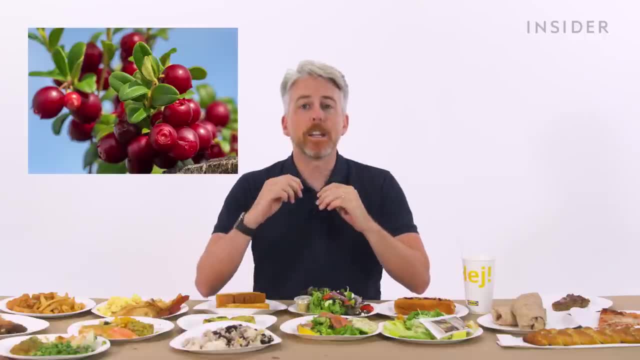 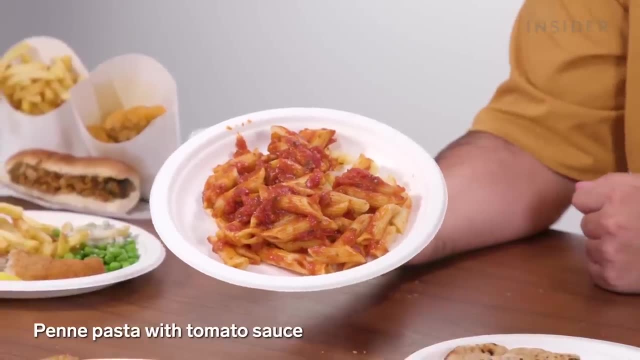 also not available at time of filming this Now. lingonberries are majorly popular in Swedish cuisine, and you're going to see them pop up a few more times in the IKEA menu. Next up is penne pasta with tomato sauce. 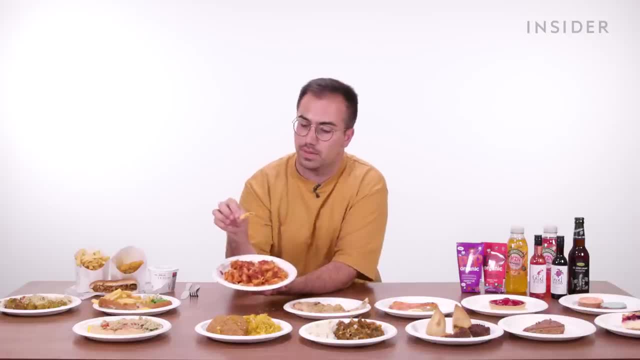 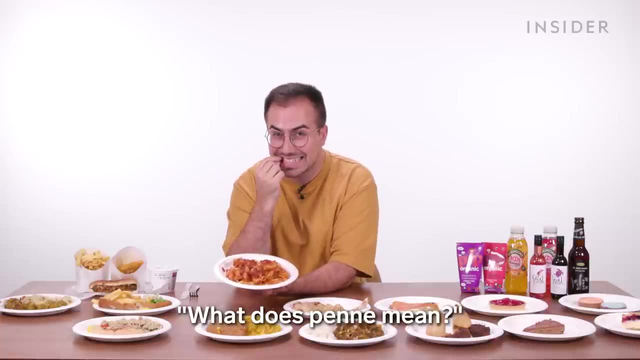 Penne, of course, refers to the shape of pasta that they use here in IKEA. Charlie's loved that. That's really weird. Is that the only analysis you're going to give? What does penne mean? It refers to the shape. 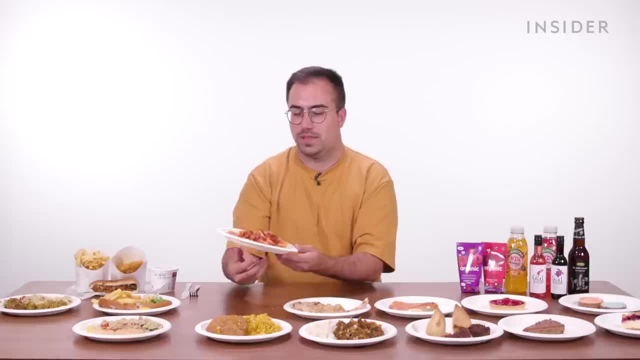 It's a string way of describing the shape, Is it? That's the shape? I think penne is majorly popular in Sweden. It may be my least favorite pasta shape. I do not respect penne Moving swiftly on from the penne. 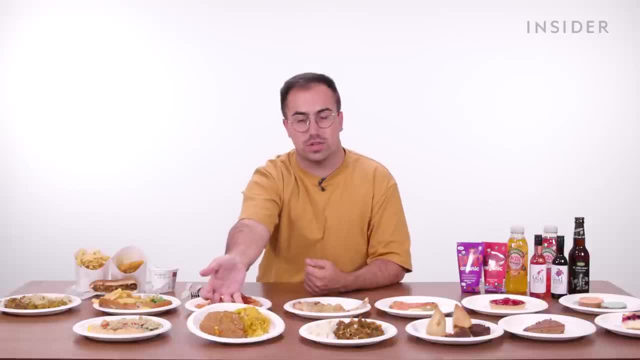 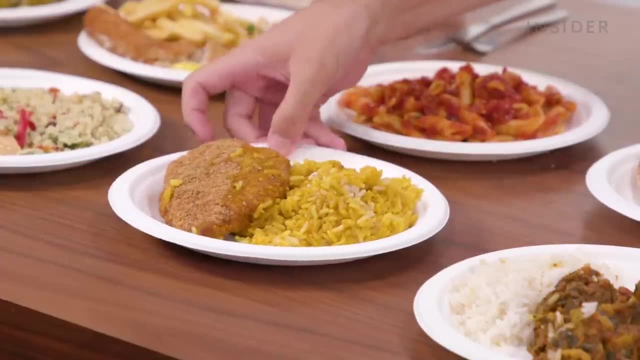 we have a chicken katsu curry. I think this is like a relatively new addition to the UK IKEA menu. So katsu refers to the chicken katsu fillet, which is a breaded and fried piece of chicken and then it's served with rice and katsu sauce. 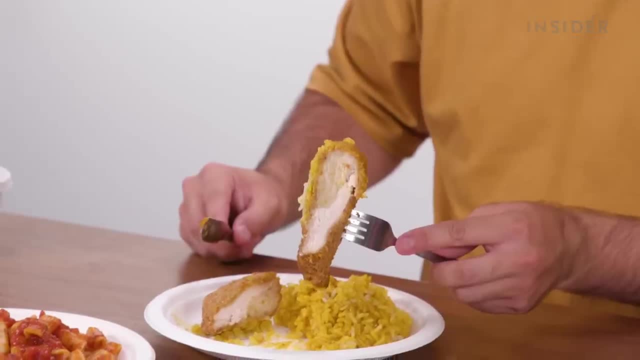 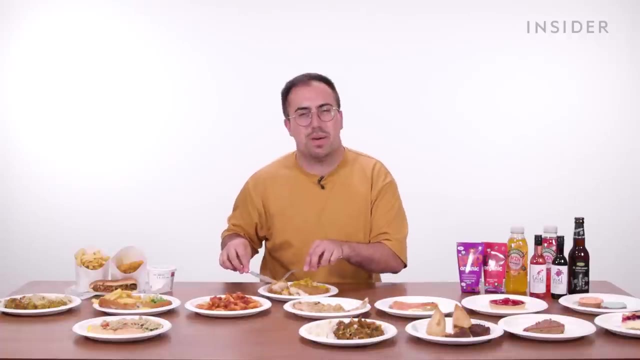 I've not tried this before. That looks like one just massive piece of chicken, you know, Oh, why are you eating it? Science, Other than a couple of like slightly disconcerting dark patches inside the chicken breast. I think it's a good idea. 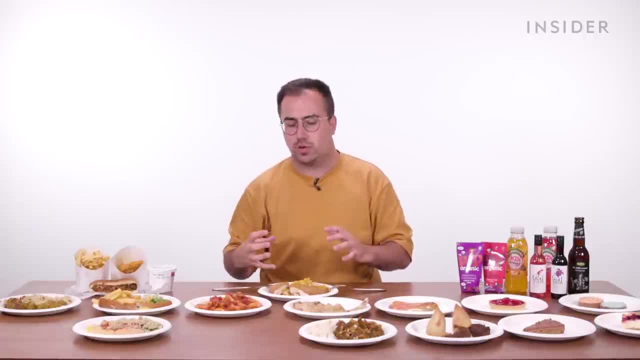 It's actually not bad. I think because of the size of the breast it's dried out quite a lot. but the katsu sauce is really nice. I like it with the rice. I think, particularly if we're eating this hot, this actually would be pretty good. 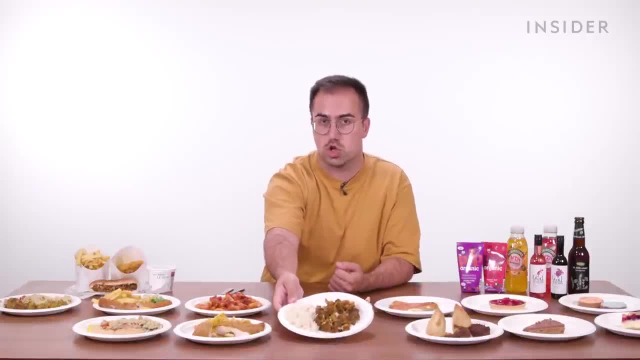 Next up on the UK menu you can find a potato and cauliflower Rogan Josh curry. A Rogan Josh is a curry that you'll find on the menu of a lot of UK curry houses. It's not super spicy, generally quite mild. 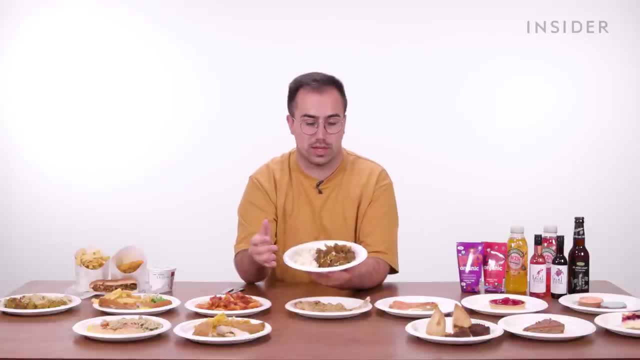 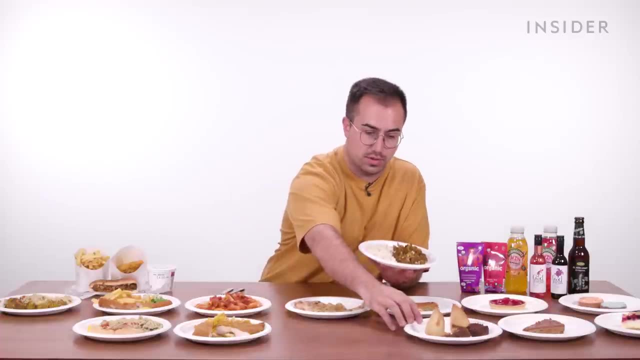 I'd say, traditionally you would see this made with lamb, but they've made a vegetarian version here, obviously with potato and cauliflower as the main bulk of it. The Rogan Josh from IKEA is served with rice, And then you can also get some side options. 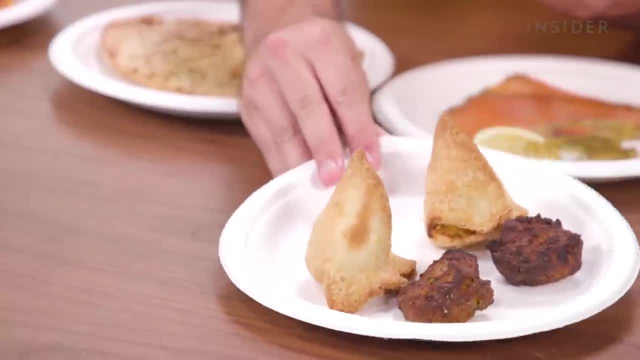 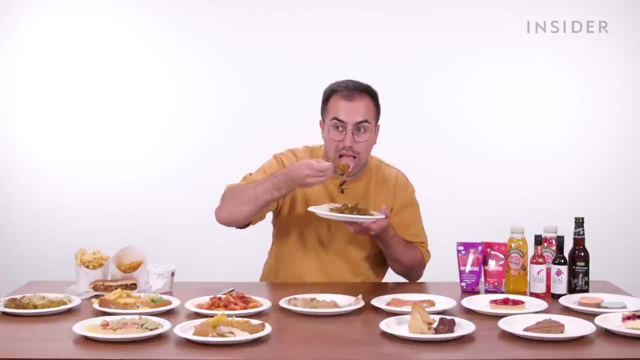 which are designed to go with it, including some pakoras, samosas and a garlic naan. Obviously, the UK has a large British Indian population, So I do think this is another attempt to kind of localize the menu. That's pretty good. 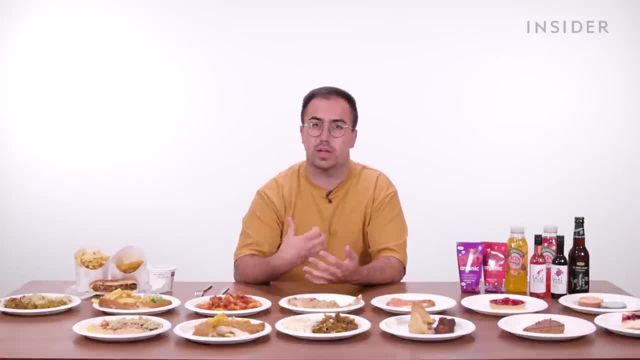 That's pretty flavorful. There are some other main course options from UK IKEA's which unfortunately we couldn't find today. These include such things as butternut squash and sweet potato soup, Mangalore chicken curry, butternut squash, blue cheese and caramelized onion pie. 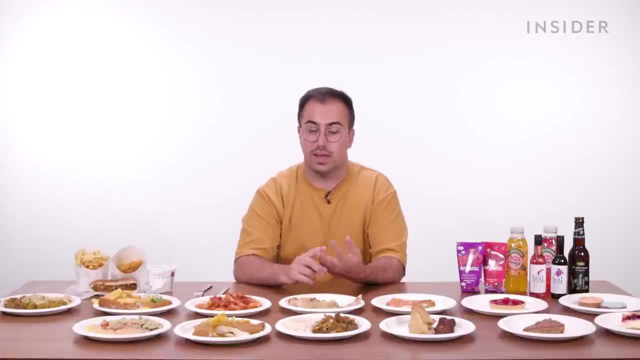 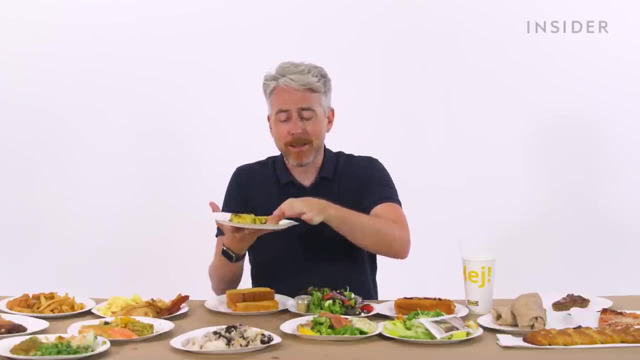 chili, sin carne, garlic butter, chicken pie and leek and potato soup. I would like to move on to sides. Right here we have the vegetable medallions. I like veggies presented like this, just like in a little puck: just bite into it. 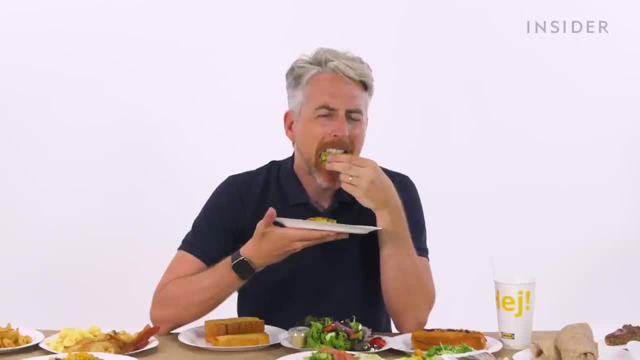 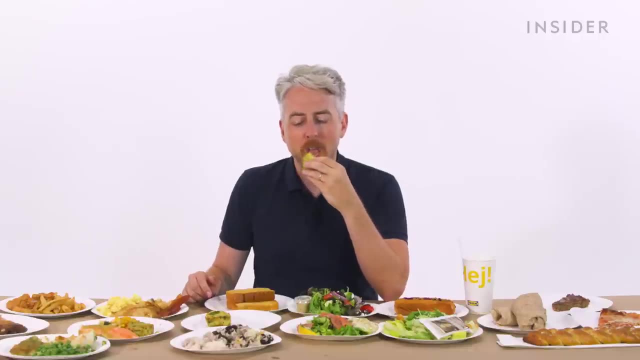 Looks like it has some broccoli mostly potato friendly Little onion, Yeah, not bad decent side. It's like you know. it's like broccoli potatoes, like broccoli mashed potatoes- The Havana chicken that I mentioned earlier. this is the beans and rice it comes with. 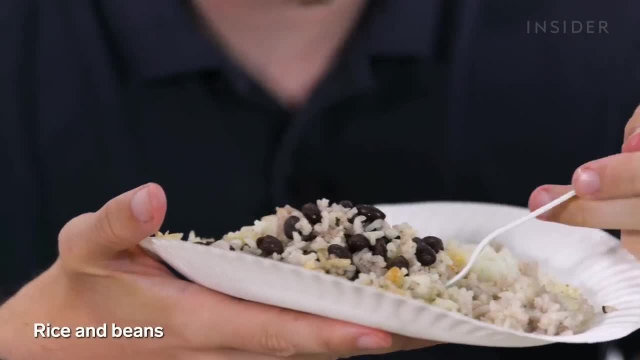 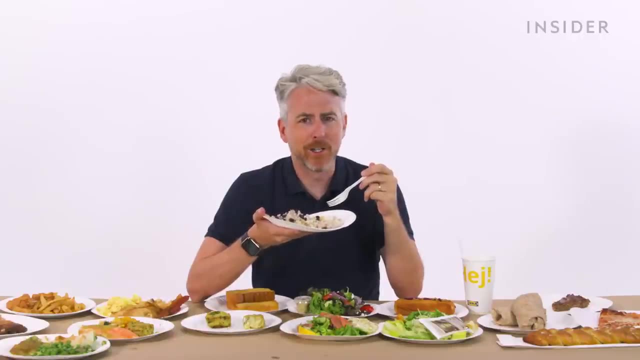 I don't know if they mix them up or just got mixed up in transit. but no beans and rice, let's go. This is just white, white rice and black beans. Like I don't taste any additional flavor to this at all. 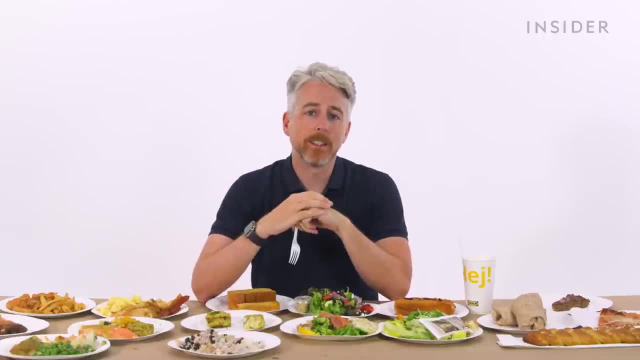 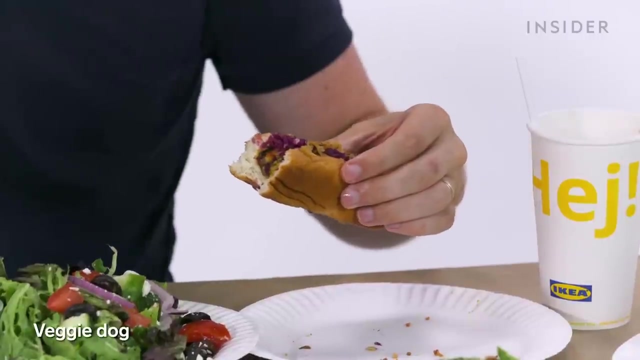 They do sometimes offer plantains Again. the IKEA we went to today did not have plantains, but they did have a garlic bread. I think that's an exclusive Onto the IKEA cold dishes. They have a veggie dog. 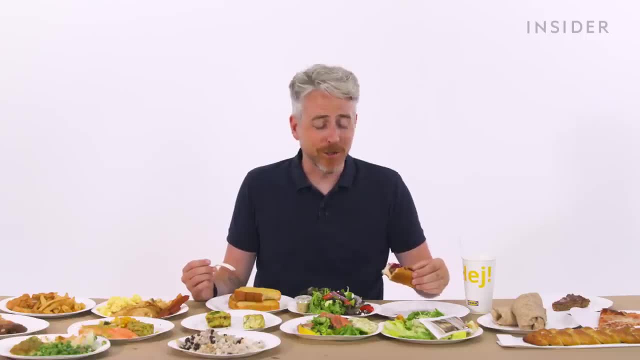 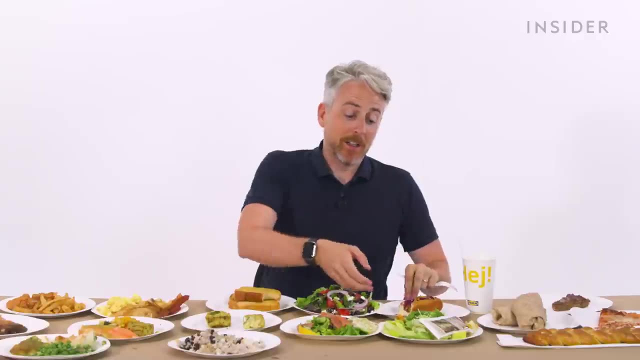 Well, the veggie dog wrap is under the cold dishes, according to the script, And this veggie dog is cold. Maybe it's been sitting a while. Either way, it's not very good. Also, they have a Greek salad, Also the Caesar salad, which, once again, 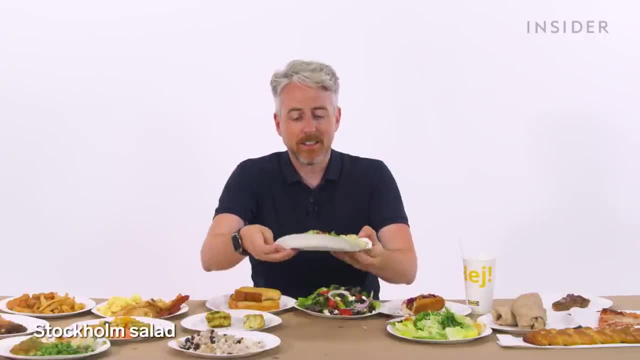 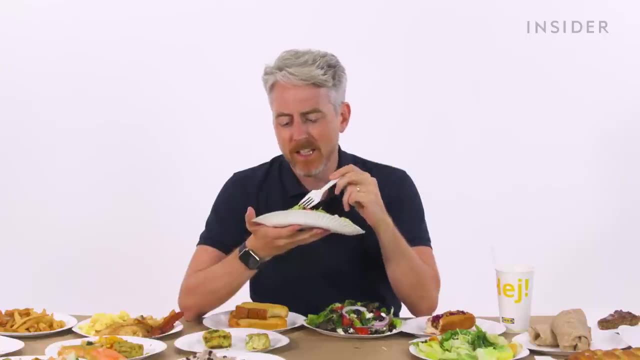 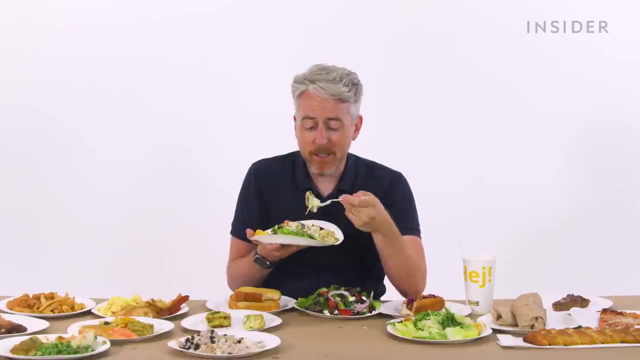 I mean, this is a pretty low effort. A Stockholm salad, Not to be confused with Stockholm syndrome, which I'm starting to feel right now. eating this food- Salmon, lettuce, lemon Sure- That's not bad actually, I like. 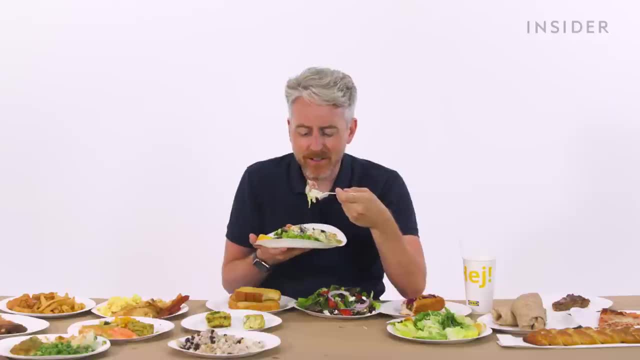 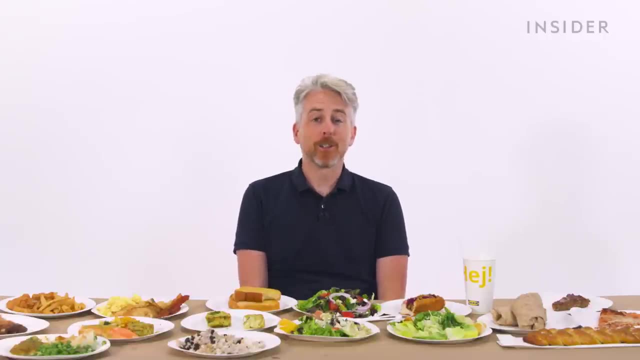 This sauce that's turning color under these lights, and this salmon. We're not quite sure what is in this salad with the sauces right now, but through the miracle of editing we can put that on the screen right, And that's what it is. 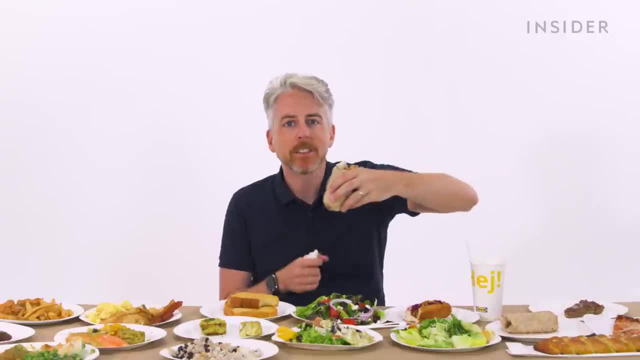 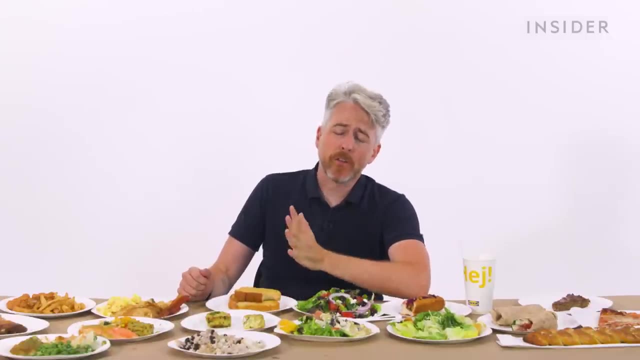 Tastes pretty good. Also, you can get a BLT chicken wrap- Not bad If you like wraps and BLT and chicken, Also at a US IKEA, which was not available at time of filming this at our Burbank IKEA. 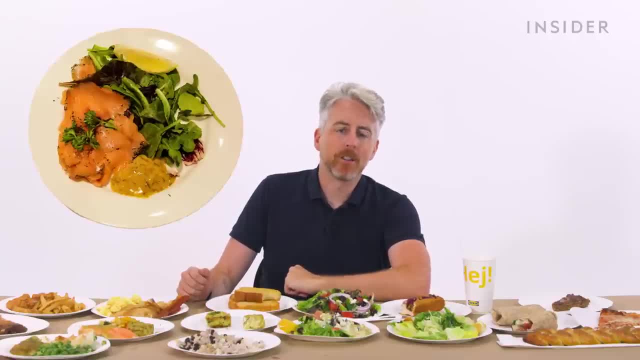 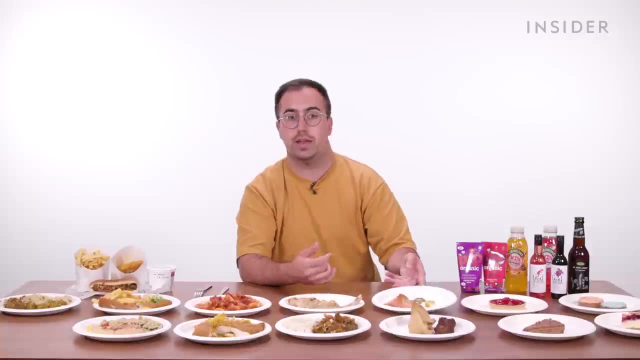 Is a Greek veggie ball wrap and marinated salmon. The UK's cold plate menu is pretty bland in comparison. The only one they had today was this marinated salmon plate, but we can also get an egg and shrimp sandwich with mayo. marinated salmon wrap. small salad bowl. 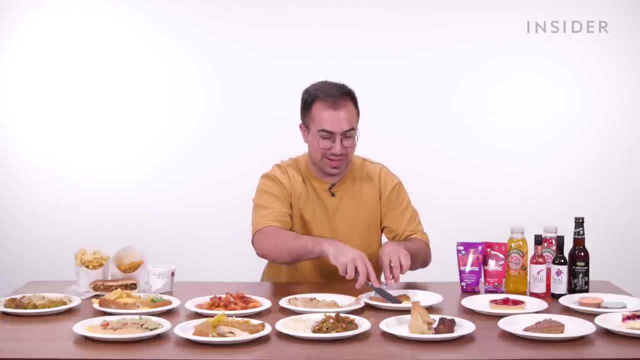 and a tomato and mozzarella salad. I guess I'll give the salmon a quick try. I do like smoked salmon Here. of course they call it grablachs because it's the traditional Swedish way, And it comes with a dill sauce and some lemon. 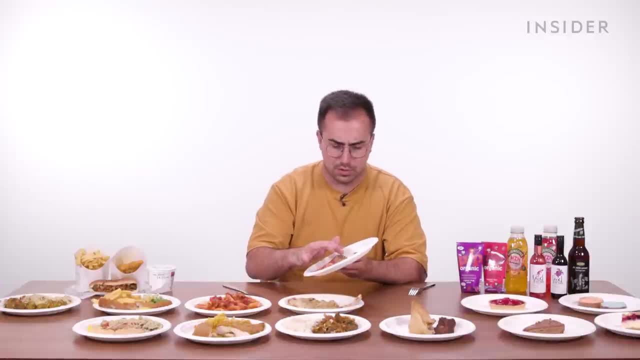 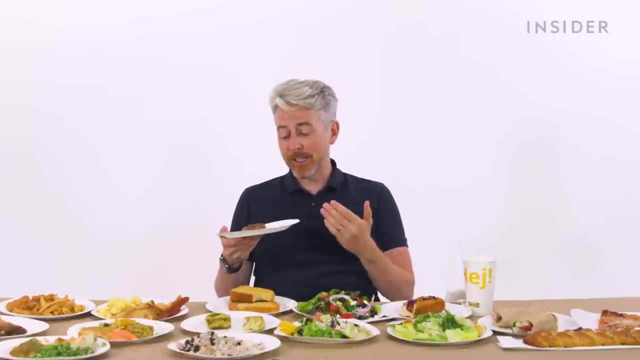 Fairly mild flavor. I like the kind of herb crusting that you get. The dill sauce is pretty dilly. And now onto desserts. There are three exclusive IKEA US desserts. I was only able to get one of them, So the first would be the strawberry shortcake. 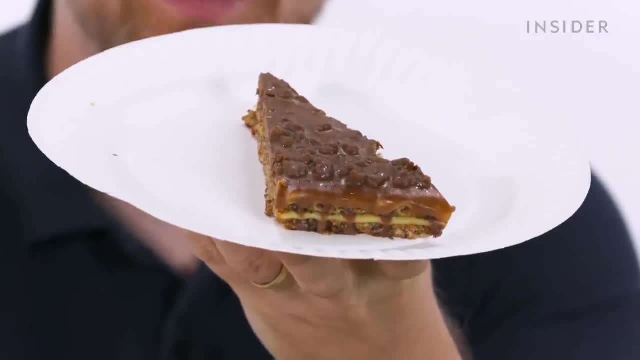 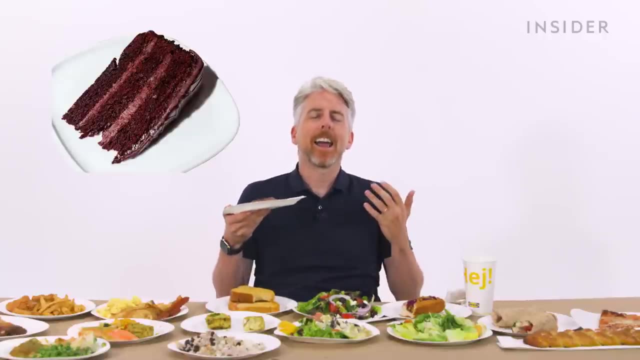 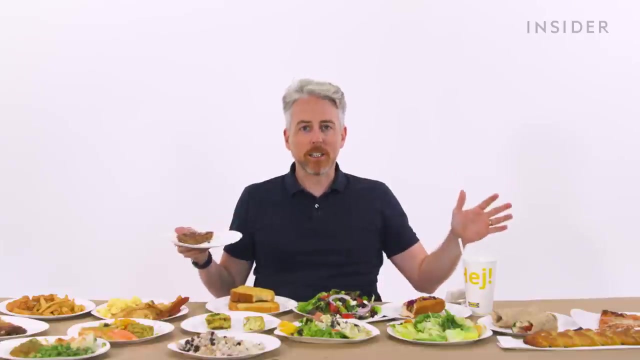 Not available at time of shooting this. The second is this, the caramel almond cake, And the third is the infamous chocolate layered cake, also known as the conspiracy cake. I asked everyone there, please tell me you have chocolate cake? And they all said no, no chocolate cake. 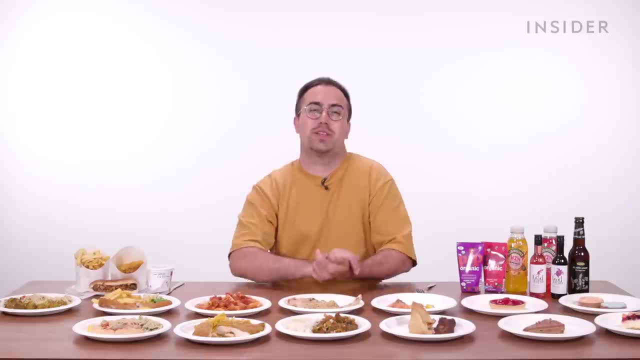 At the Burbank IKEA. today at least Tragically, we don't have the conspiracy cake here in the UK. but we do have some other exclusive dessert options, For example this delightful looking strawberry tart. There's some real pieces of strawberry in there. 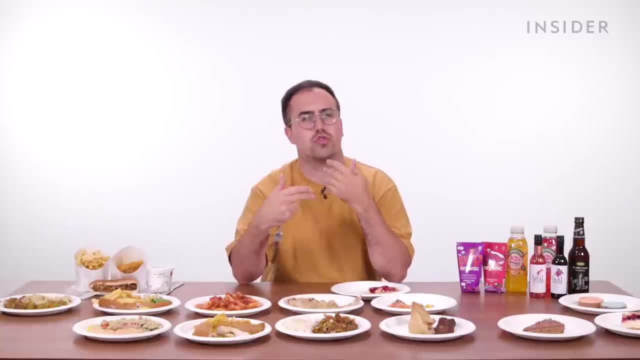 I like the pastry, I like the cream, I like the fresh strawberries- Whatever the kind of strawberry syrup, jelly stuff that they've kind of put around the outside is, it's okay, But it has like a slightly almost like medicinal quality to it that I don't really love. 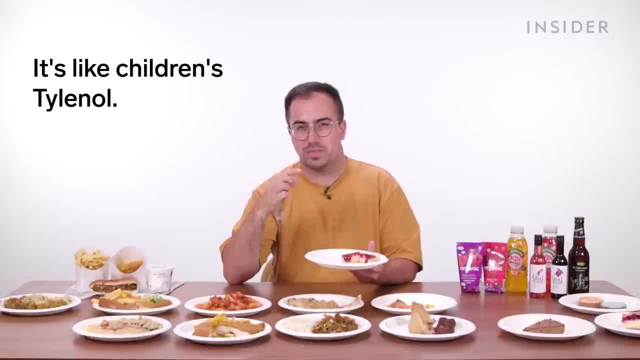 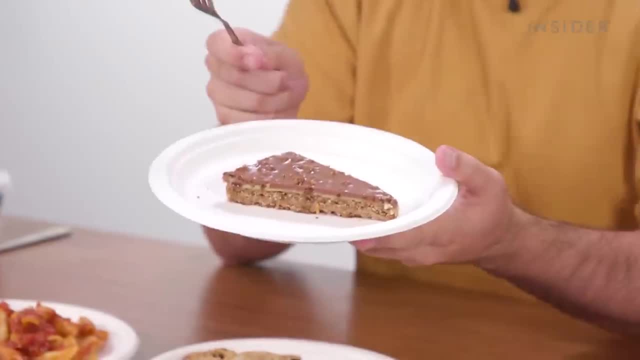 It almost reminds me of a Cal-Pol. I don't know if you have that in the US, but it's like a medicine. It's marketed towards children in the UK. Next up, we have IKEA's famous dime cake. Now you do have this on the menu in the US. 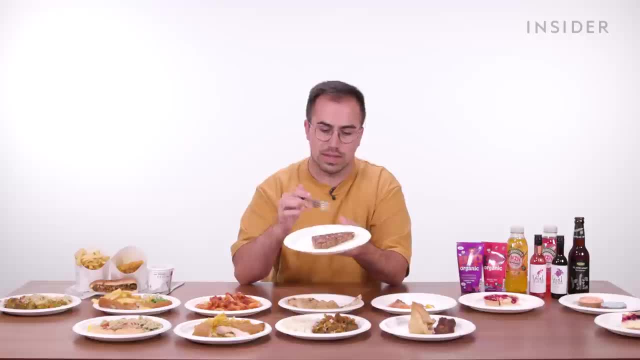 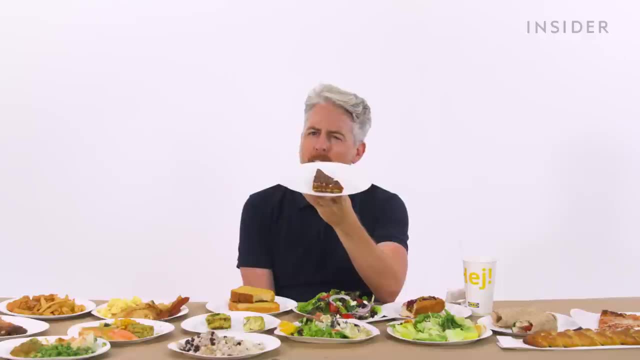 However, I believe you guys call it something slightly different. I think caramel almond cake. Is dime not a particularly big brand name in the US, Because over here in the UK I'd say most people are familiar with dime as a chocolate brand. 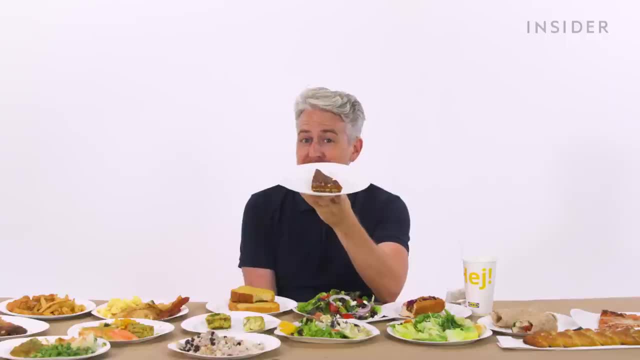 Harry was just talking a minute ago about the dime cake, the DM cake, D-A-M cake. I've never heard of it. I've never heard of that brand. I have no idea what it is. I'm sorry, But we do have this. 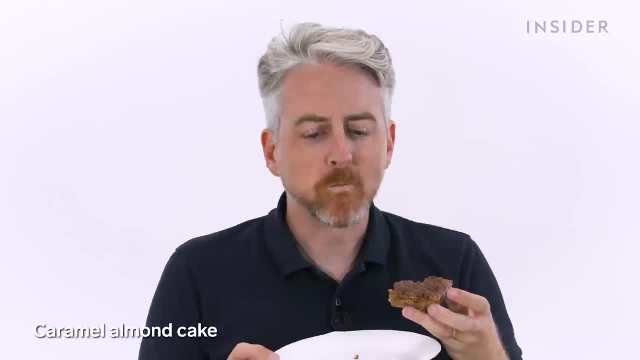 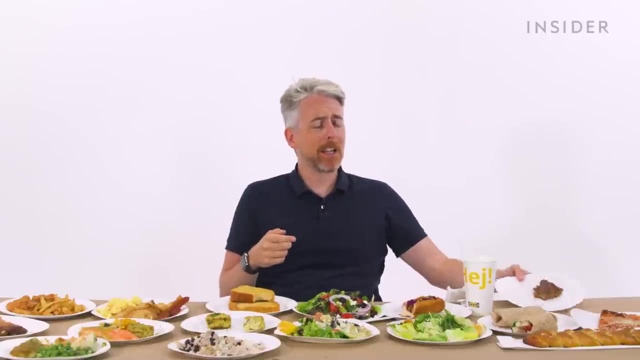 which I think is supposed to be similar. Oh yeah, This is fantastic. I'm getting one of these every time I go. I'm gonna get one of these and I'm gonna get that chocolate cake. I'm gonna be on lookout for it now. 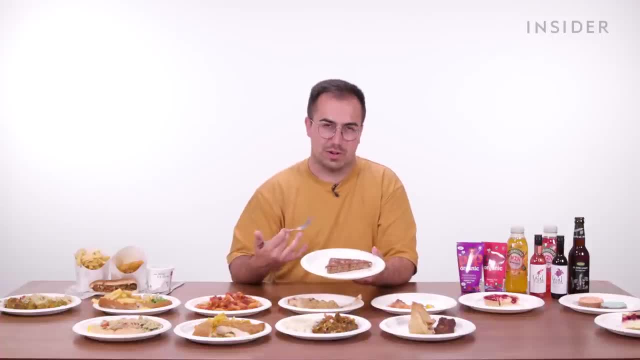 It's maybe not quite as popular in the UK as it used to be. It reminds me of my granddad a lot because he used to really love a dime bar. I wouldn't see many people my age going for it, but still very tasty if you're in the mood for it. 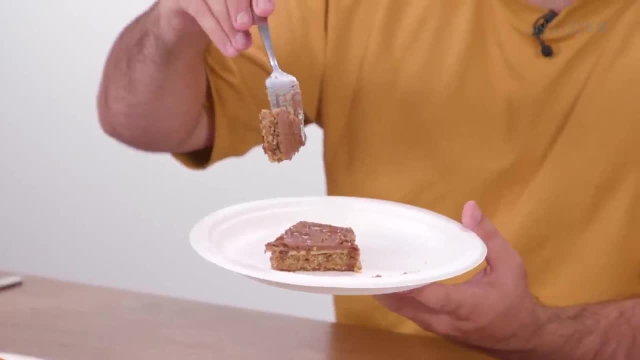 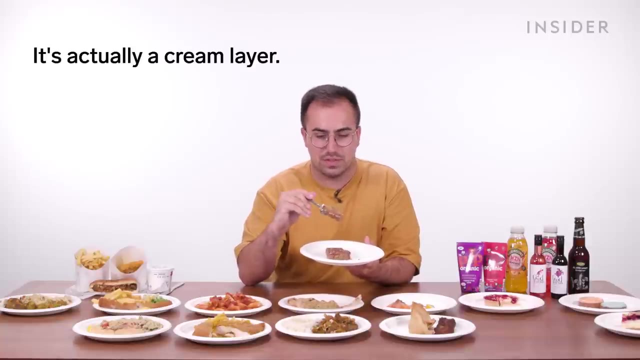 And this cake is sensational. You get these layers of chocolate, this kind of biscuity crumb and these kind of- like I thought, all these pancakes in the middle. I think these dividing lines might all almost be kind of cold chilled pancakes. 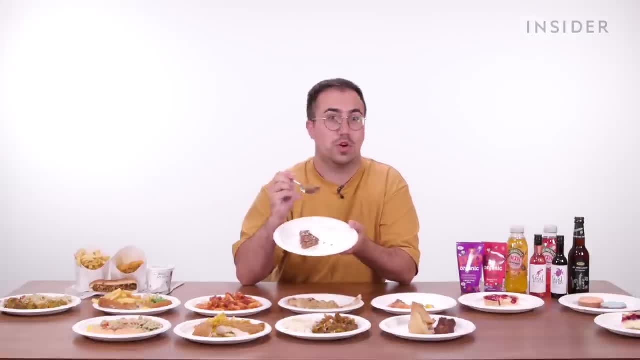 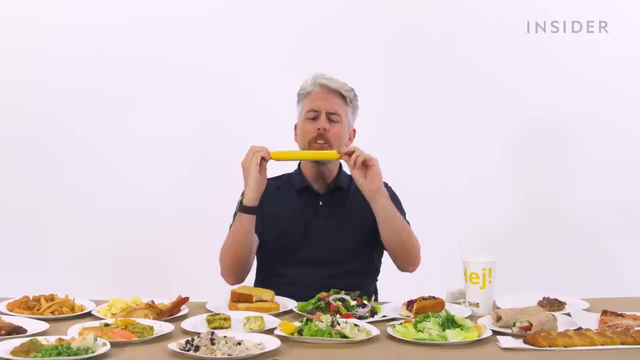 This might be my favorite thing on the menu. This is why I'm making excuses to go to Ikea. Hmm, They did have these at the register and this also says dime on it. Have you seen that? Yeah, okay, This tastes like this. 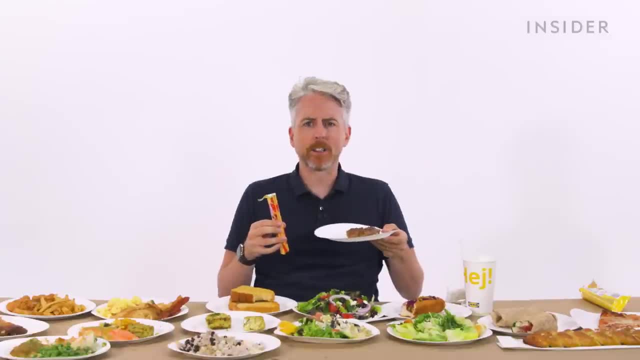 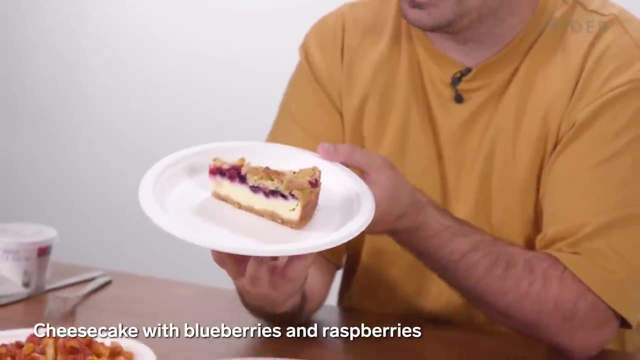 Never heard of this, but it's very good And this is fantastic. I maybe just rebranded it because no one in the US knows what dime cake is. Our next dessert option is a cheesecake with blueberries and raspberries. 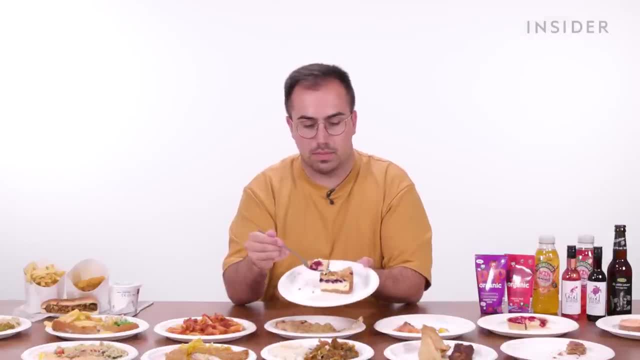 It's a very soft cheesecake, really like easy to cut. There's like a nice baked crumb. on top There's a layer of the berry stuff, So there's some blueberries in there, some raspberries, Then finally we have these. 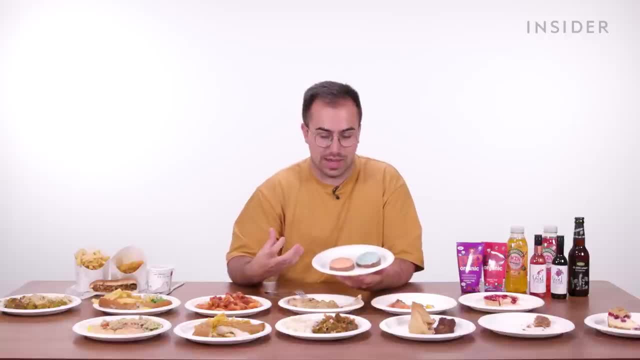 under the sea. rocky road biscuits. Obviously, rocky road in the UK is a dessert which is usually like a no-bake dessert, made of things like melted chocolate, golden syrup, marshmallows, even things like corn flakes, pieces of biscuit, that sort of thing. 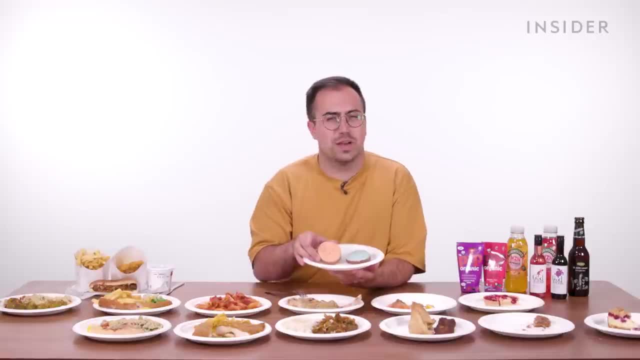 All just kind of mixed together, left to set, and then you have a nice easy dessert. It turns out. what makes this under the sea is that they have a kind of animal stamp in icing on top of it. Here we have this nice octopus. 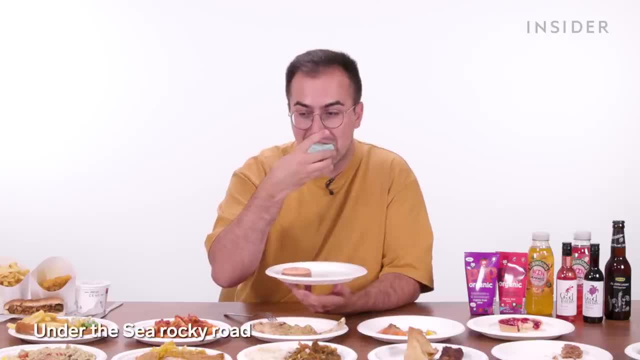 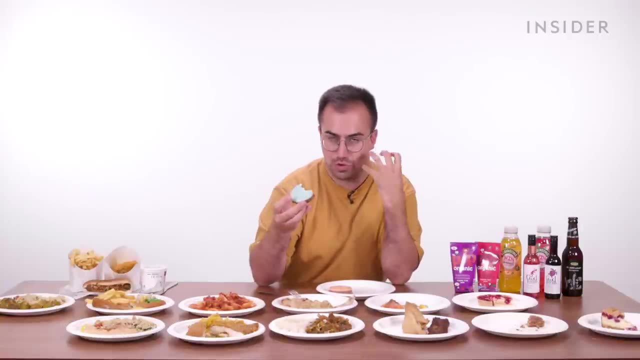 and here we have a couple of dolphins. I think when I eat a rocky road, I kind of want some more distinct elements. I like being able to bite into it and crunch through a bit of biscuit or chew through a raisin or something. 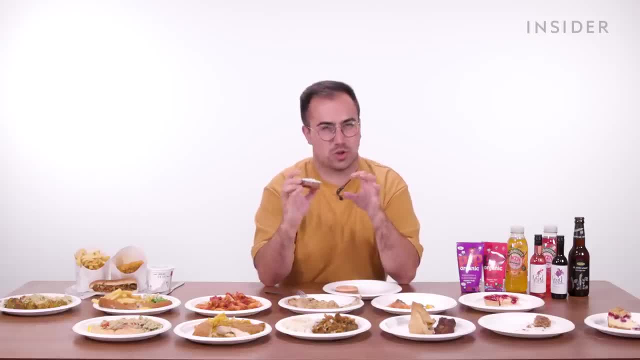 Whereas with this one it's kind of all blended together So you don't really get the like texture contrast. The flavor is very much there. It's still all those elements that I'm used to in terms of the flavor. You may also be able to find some other dessert options. 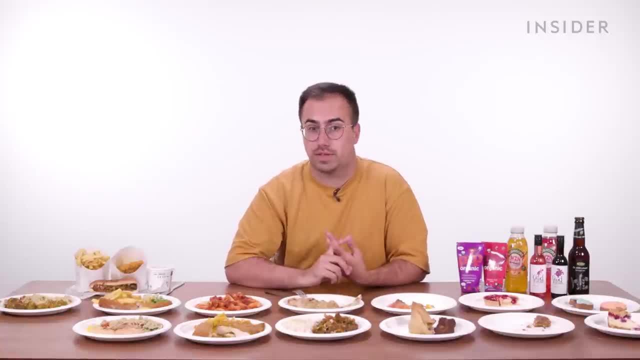 on a UK menu which we couldn't find today. These include things like a caramelized biscuit cheesecake, a chocolate clementine bomb, an elderflower and lemon cake, a gooey chocolatey cake, a lemon cheesecake, rhubarb and custard cake and a strawberry jelly. 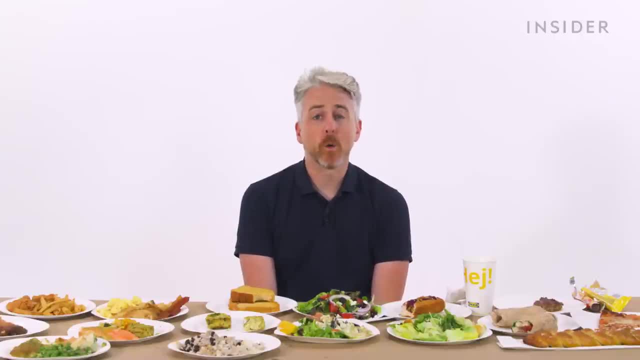 Aside from its restaurant, IKEA also has the Swedish Bistro for quick bites. The Bistro serves quick bites like hot dogs and pizza slices that you can generally grab on your way out of the store. Few exclusives we had, of course, was pizza slice. 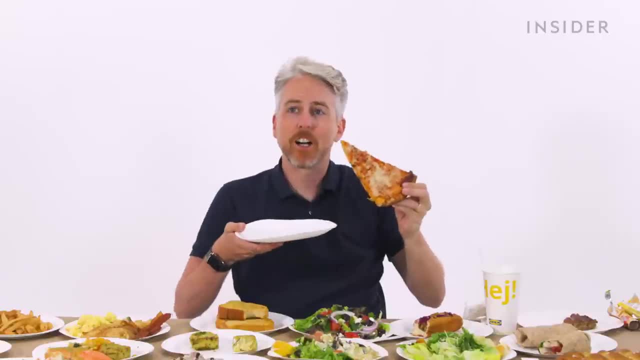 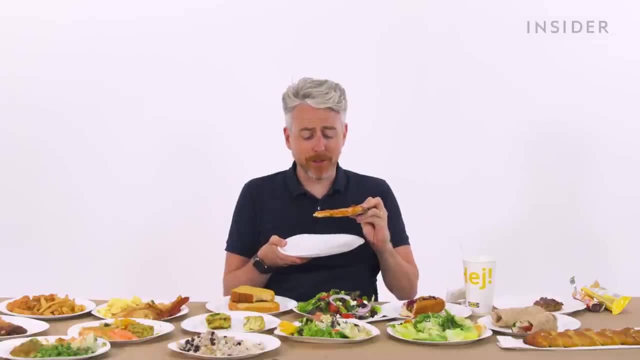 There it is, That one with cheese. Is this like Costco? or like, surprise, IKEA has amazing pizza? This is a really good slice of pizza. I can't tell, but I think this was oven cooked- Fire oven cooked, not just like the pizza. 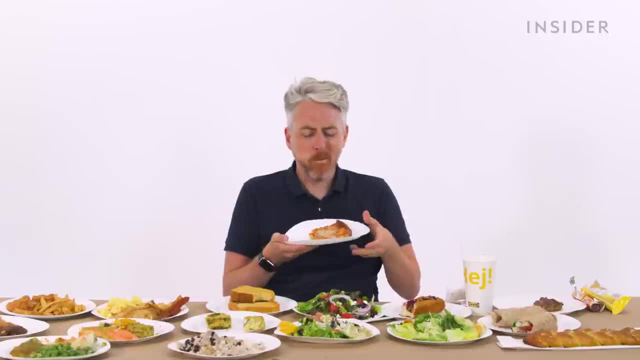 This has like a- yeah, there's a brick oven. It's not as good as Costco, but it's pretty good. Wow, weird IKEA's got good pizza. Good on you, IKEA, You can also get this giant Bistro pretzel. 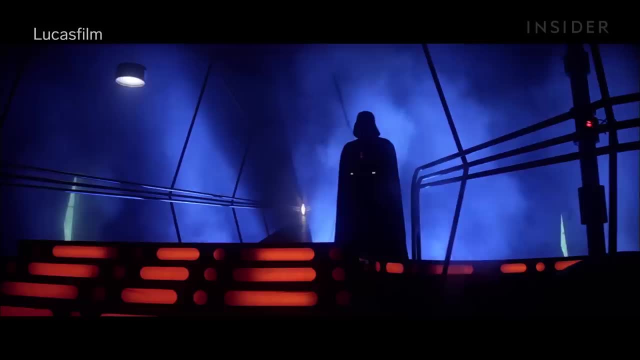 Oh, it has all it has, like a little braid here. Look at me, I'm a Jedi, But you are not a Jedi yet. And it comes with mustard. They didn't have the mustard either, man, I don't know. 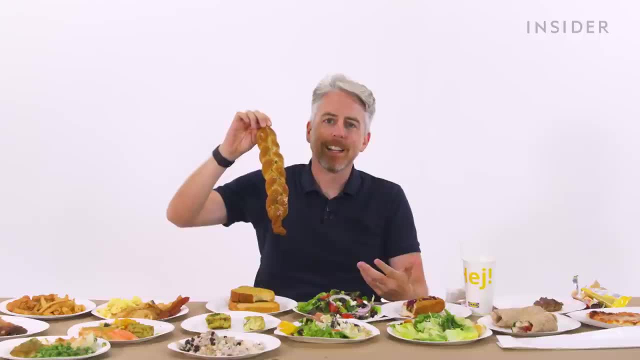 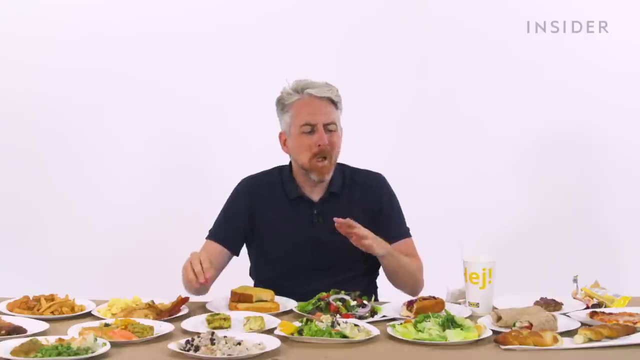 Is it because I went at 1030 in the morning and the stuff hadn't shown up yet? They didn't have anything. A pretzel with no mustard? Oh no, This is a different stuff. Also, the US IKEA Bistro. 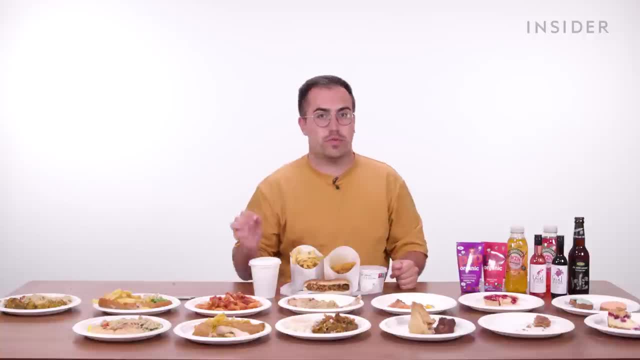 you can get a marinated salmon baguette. They didn't have it. We have a few exclusive Bistro options of our own in the UK. Firstly, if you like the onions on the hot dog, you can just get a side of fried onions. 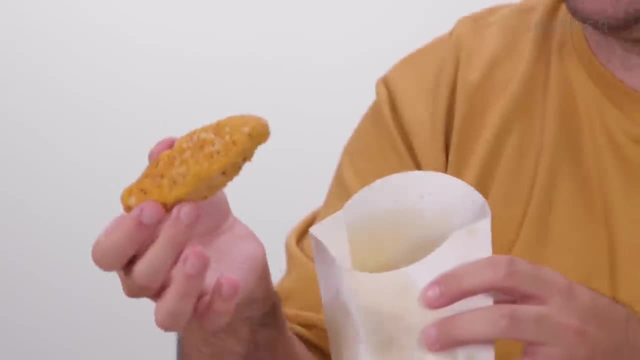 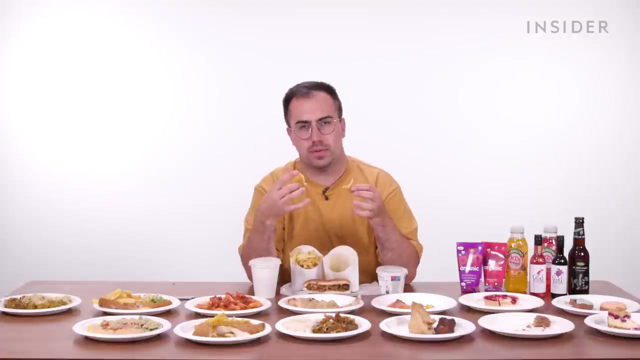 Next up we have these, which are chickless strips, So these are a plant-based version of a chicken tender. I'd say they look pretty good. They kind of passed the visual test. Yeah, when I tore this apart I was worried that the texture wasn't going to be right. 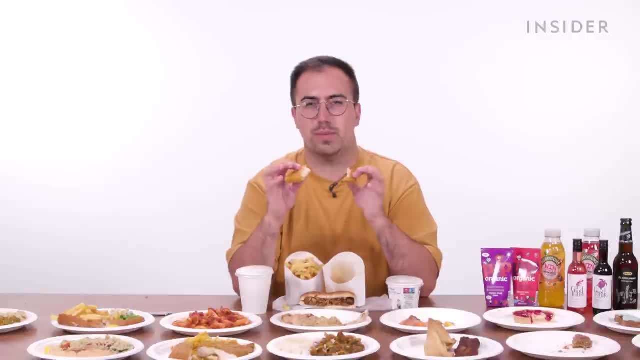 And unfortunately it's not. It's very spongy, It's very mushy, It just needs a little bit more texture, Just like to make it resemble a chicken tender a little bit more. Obviously, when you get an actual piece of chicken tender, 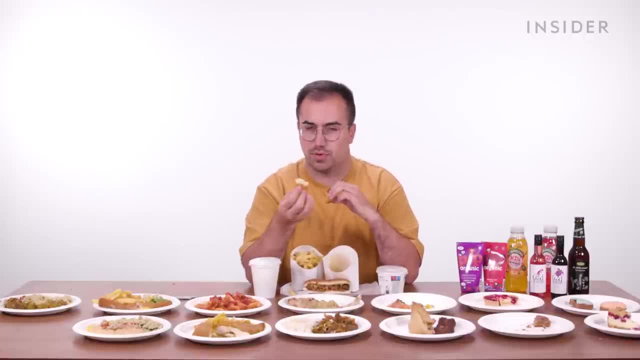 or chicken breast. you can kind of tear it and you see those strips and the fibers. They just really haven't got that here. The flavor's not too bad, though. We can also get chips from the Bistro in the UK. It doesn't seem like you guys can do this in the US. 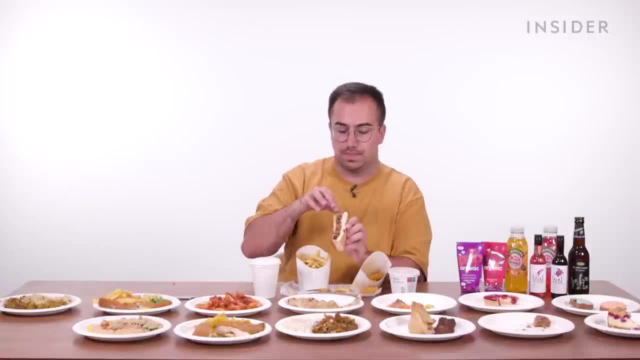 We have our veggie dog option, which comes with the same toppings as the regular hot dog. So here we got fried onions. You can also get some with pickles. The veggie dog in the UK isn't like a plant-based meat thing. 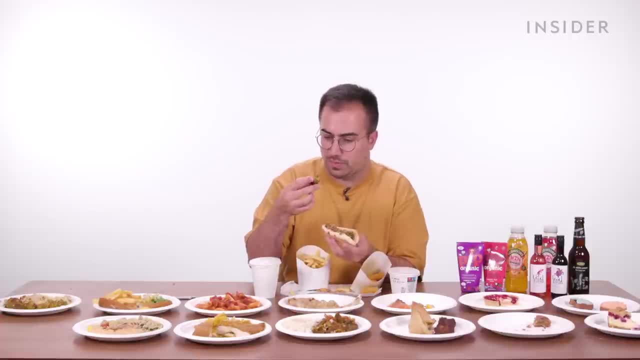 It is just vegetables, So it looks like there's some kale in there, some carrot, maybe like some mustard seeds. I think that, with the fried onions, with the pickles and some sauce, actually a pretty good veggie option. Then we have some drink options, notably milkshakes. 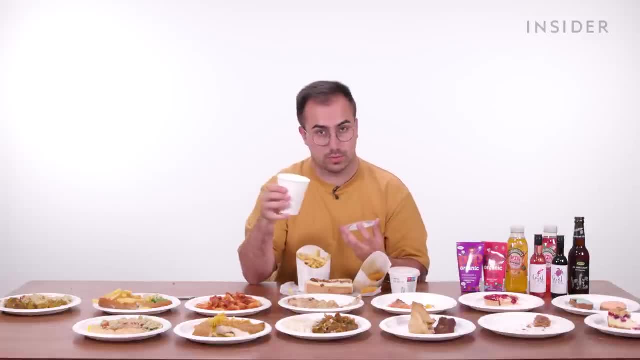 In the UK you can get milkshakes in four flavors: vanilla, chocolate, strawberry and banana. We've got a banana one today. Have a little sip. That's not bad. Pretty gentle banana flavor. It's mostly just ice cream. 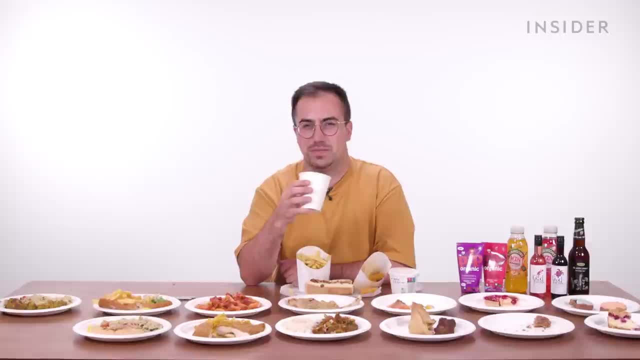 but with like a little bit of flavoring in there, which who can. who could say no? Ikea in the UK does serve breakfast, although unfortunately when we arrived today they weren't serving it. The options that you'll find there are pretty much everything that you would normally find. 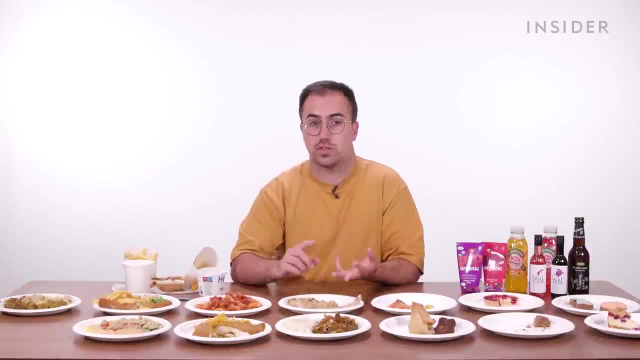 on a full English breakfast, So it includes things like bacon, sausages, hash browns, beans, tomatoes, mushrooms, black pudding- Sometimes you'll find things like that, things like patty scones as well, And you can also get white or wholemeal toast. 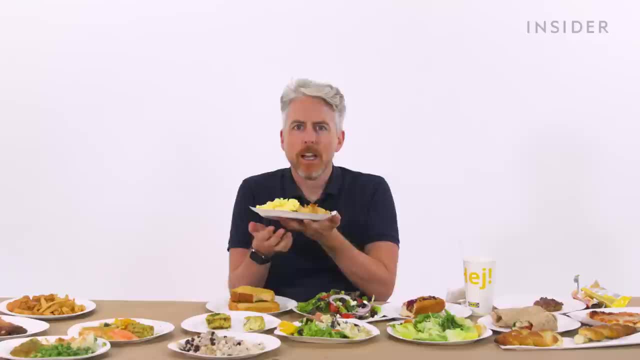 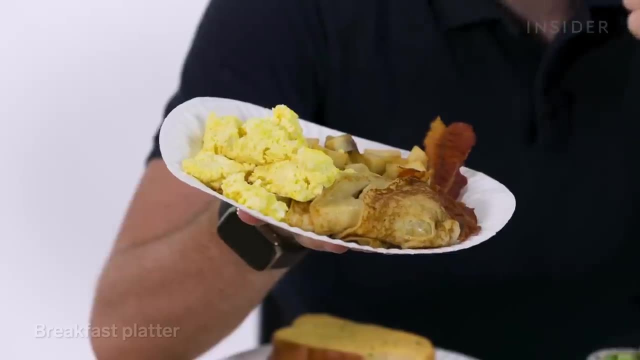 If breakfast platters aren't your thing, then you can also just go for some fruit or some porridge Breakfast. The breakfast platter in the US also comes in both regular and small sizes, and it's made up of eggs, potatoes, bacon, Swedish pancakes. 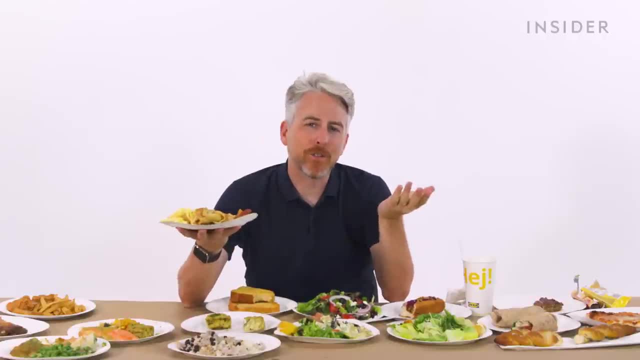 and now it's supposed to be topped with the lingonberry jam and then give it to us. The US breakfast menu also offers a Skagen croissant sandwich, which is a croissant filled with traditional Swedish shrimp salad Salad. eight and a half. 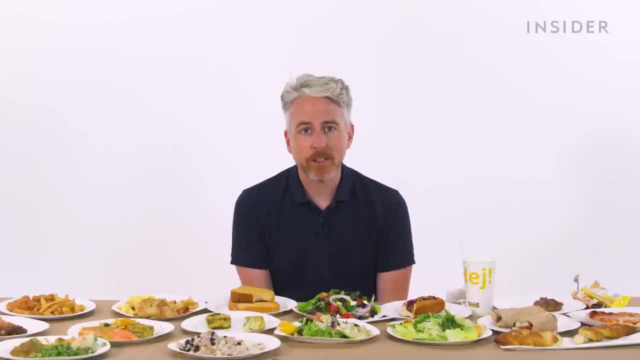 I think Ikea has its own line of drinks available in its restaurants, The US Ikea's. you'll find cola, sugar-free cola, sparkling raspberry juice, lingonberry juice and sparkling lemonade. I went ahead and got the lingonberry juice. 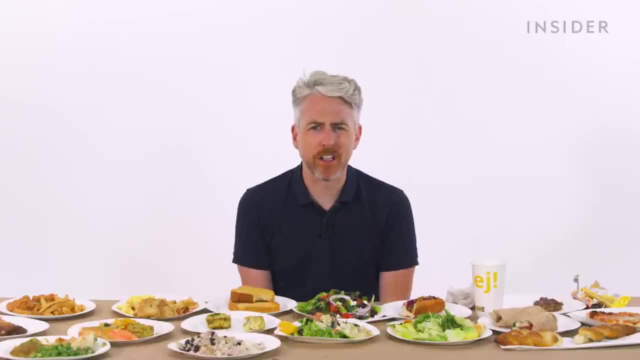 Straight up. no idea what a lingonberry is, but it's fantastic. There's no difference in the size cups. You just have glasses that are the same size or these to-go cups or whatever. We have some drink options at the restaurant in the UK. 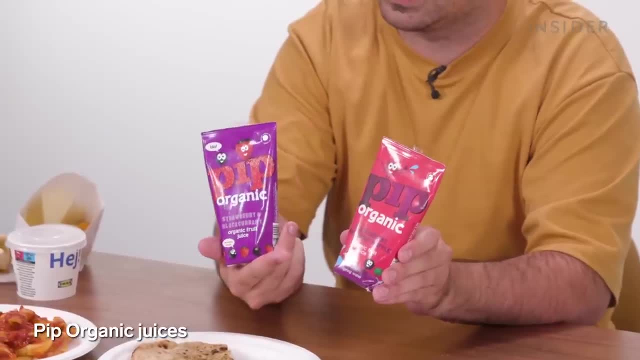 that you guys might not have in the US. There are a couple of options for kids, Which are these: Pip organic juices. We have a couple of Robinsons options in the UK. Robinsons is probably the most popular brand of squash in the UK. 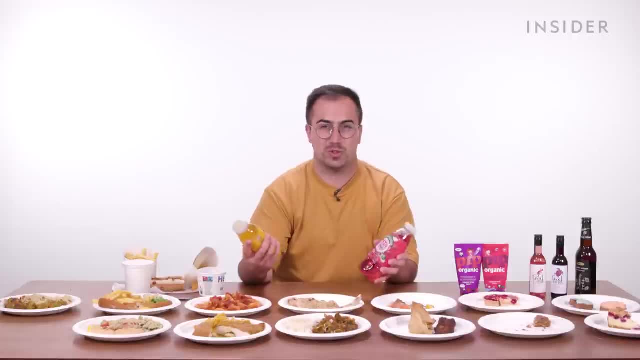 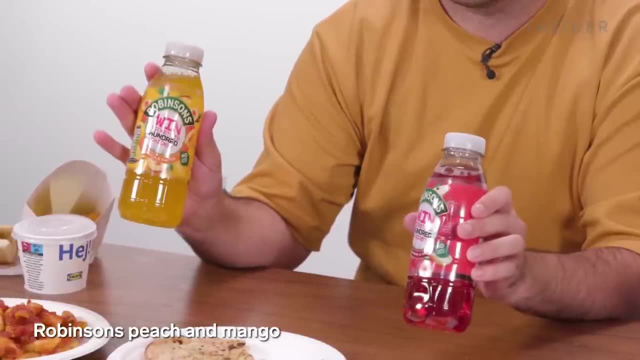 and this is basically just a diluted version of their squash. Squash, for those who don't know, is like a concentrated fruity drink that you kind of water down to have a nice refreshing beverage. You can get a peach and mango version or a raspberry and apple version. 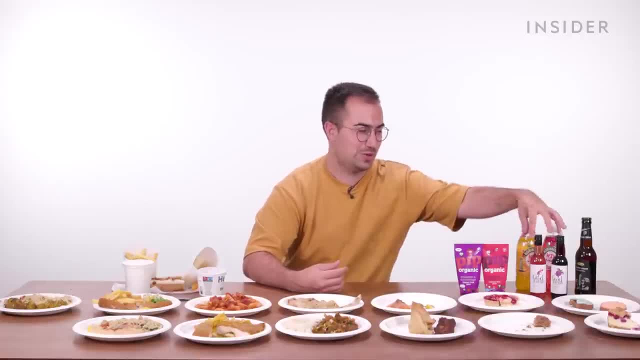 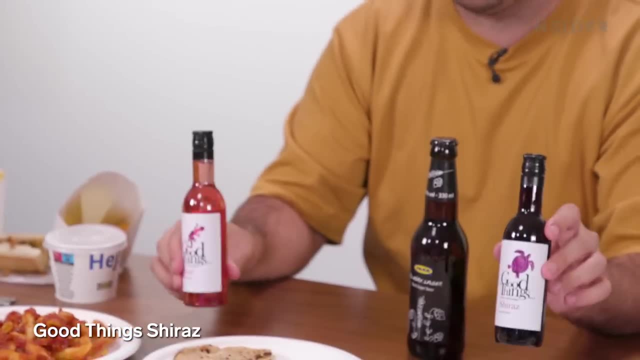 And if you feel like celebrating any of your purchases that you've just made from the Ikea, you can also get alcohol. We have three alcoholic options on the menu at the UK Ikea: A rose wine, a red wine or a dark lager. 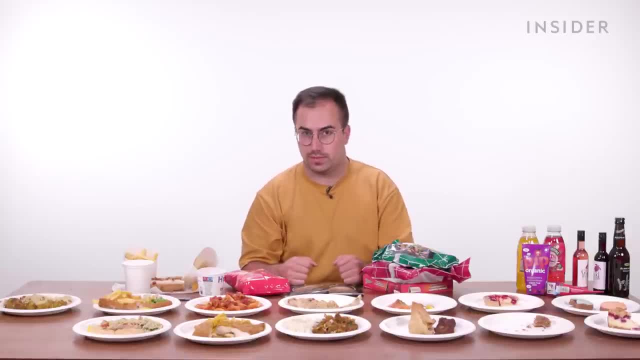 Finally, Ikea has a Swedish market where you can buy pre-packaged food items to take home. The items on offer include some of their classic foods, like the meatballs which you can buy frozen, or some gravy sachets which you can make at home. 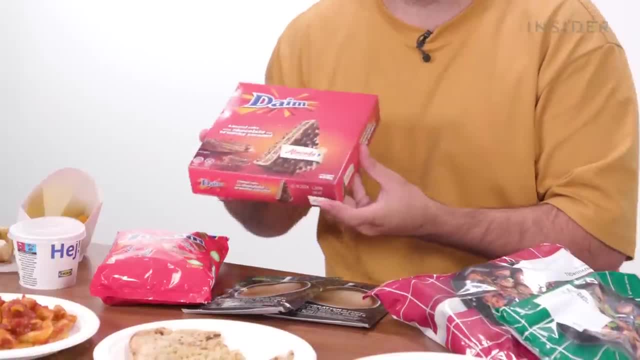 In the UK. you can also find the plant-based balls on offer. in there You can get a whole frozen dime cake which I will be taking home and eating all by myself. And speaking of dime, you can also get the chocolate which the cake is based on. 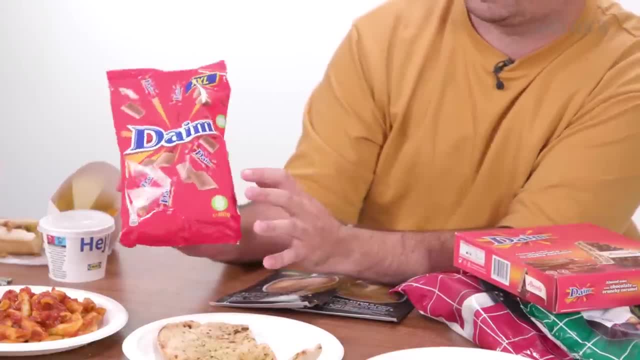 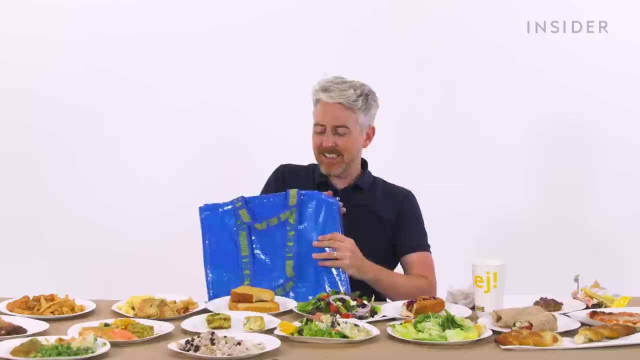 Here it's in bite-sized form rather than as actual chocolate bars, But as you can see, it's chocolate with a kind of hard caramel center. Charlie has dibs on these. Another thing at the US Ikea, Maybe not exclusive per se. 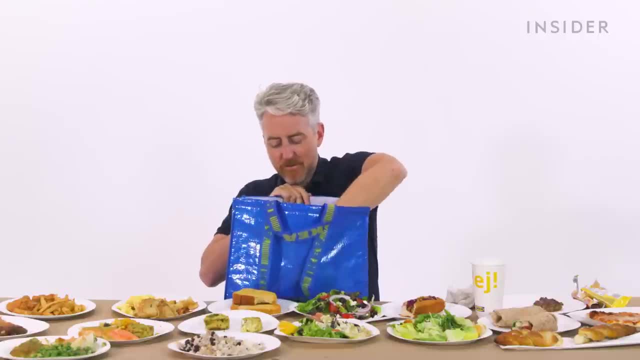 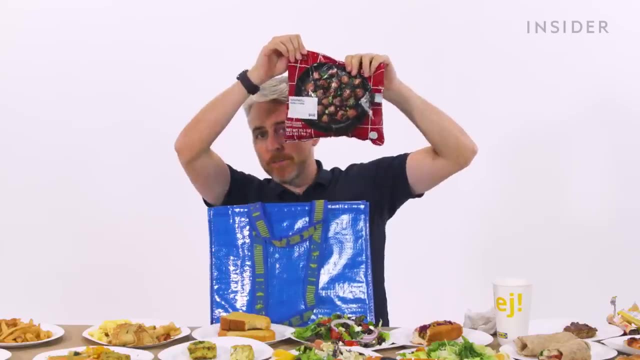 but of course they have a whole thing of frozen stuff. I had us grab stuff that was interesting. Come on the cinnabuns. huh, The cinnamon buns, meatballs. And you know, we were talking about the dime cake. 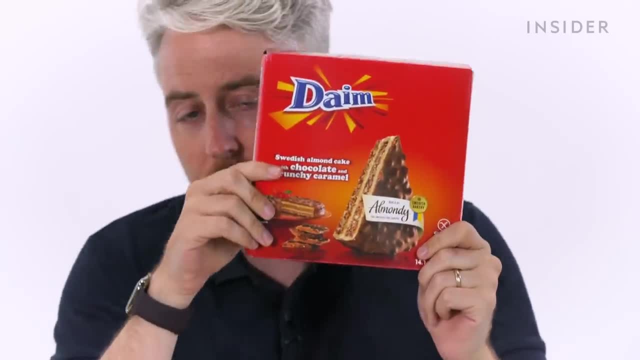 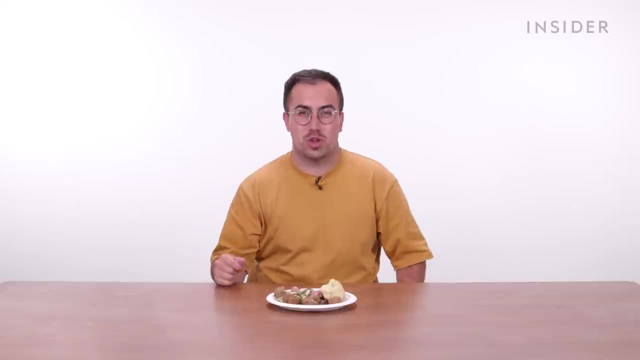 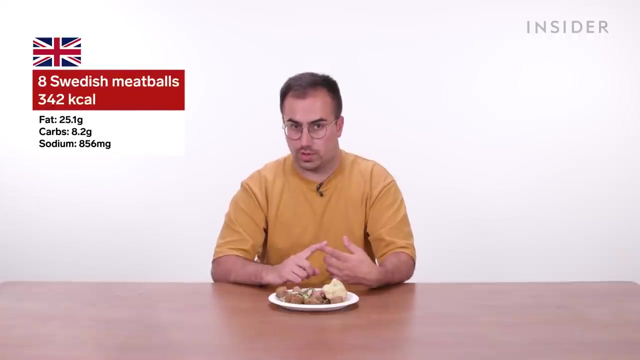 but they do have it frozen to take home And of course it is the dime cake. Let's compare the nutritional information of some iconic Ikea dishes in the US and the UK. In the UK, eight Ikea meatballs contains the following: 342 calories, 25.1 grams of fat. 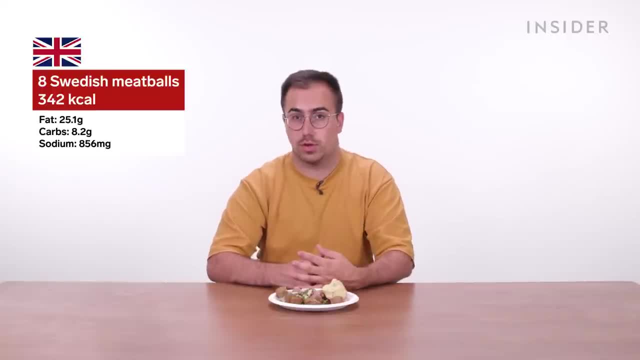 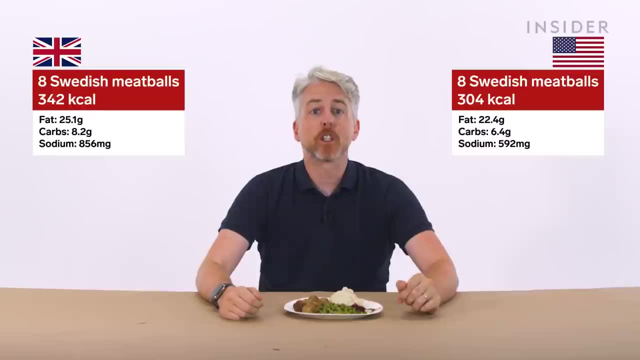 8.2 grams of carbs and 856 milligrams of sodium. In the US, the same plate of Swedish meatballs contain 304 calories, 22.4 grams of fat, 6.4 grams of carbs, 592 milligrams of sodium. 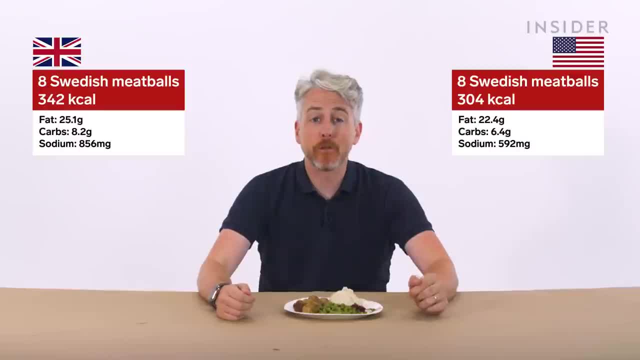 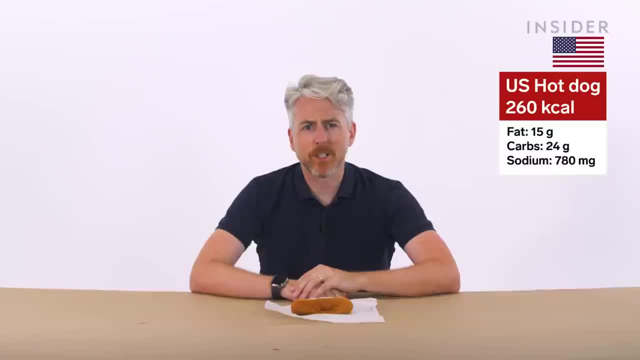 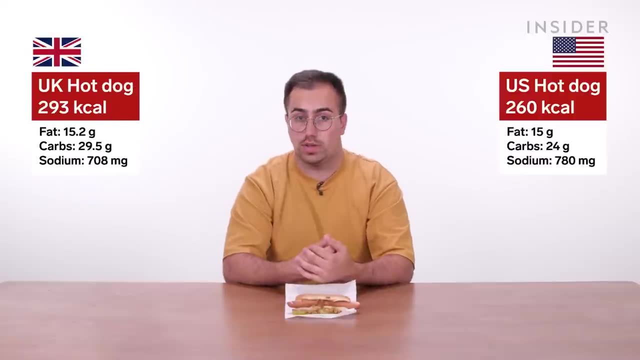 What about the Ikea hot dog? In the US, it contains 260 calories, 15 grams of fat, 24 grams of carbs and 780 milligrams of sodium. And in the UK the hot dog contains 293 calories, 15.2 grams of fat, 29.5 grams of carbs. 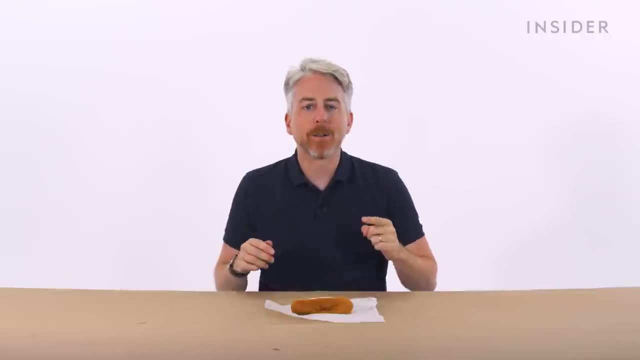 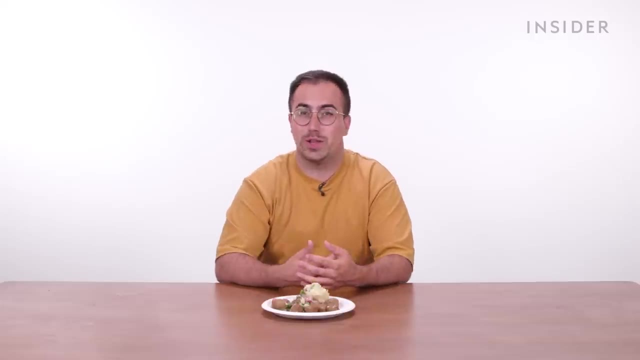 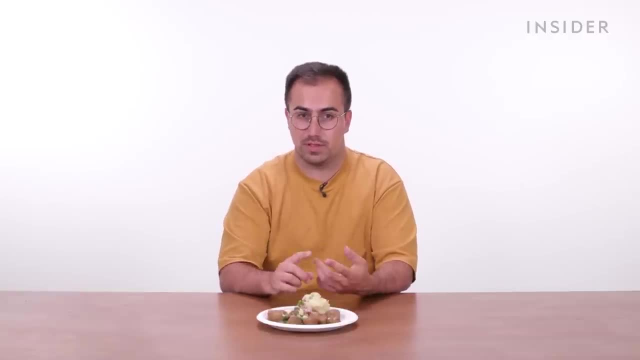 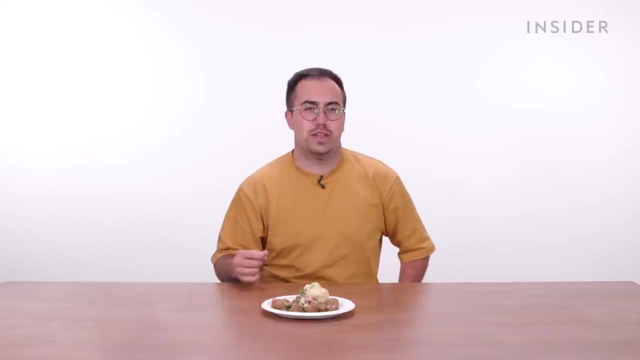 if you want to make the meatballs at home, you use the following ingredients: Beef mince, pork mince, onion, garlic, breadcrumbs, milk, egg and salt and pepper to taste. But is that actually the ingredients list for proper Ikea meatballs? 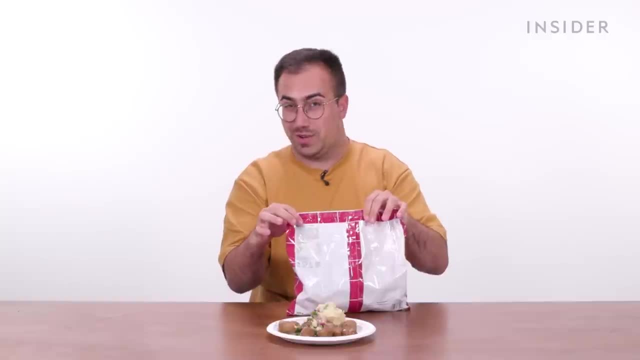 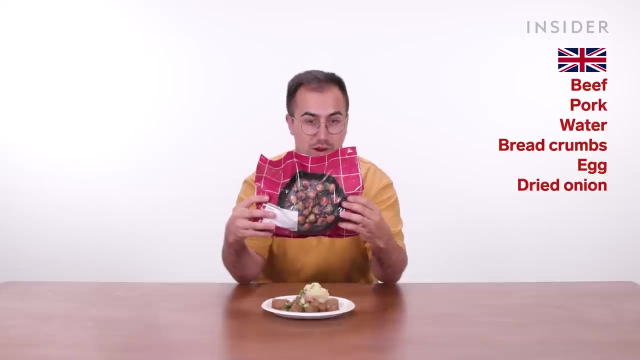 Well, on the back of the frozen packet you'll find an ingredients list. According to this packet, they contain beef, pork, water, breadcrumbs, egg dried onion, salt, egg powder, black pepper extract and allspice. 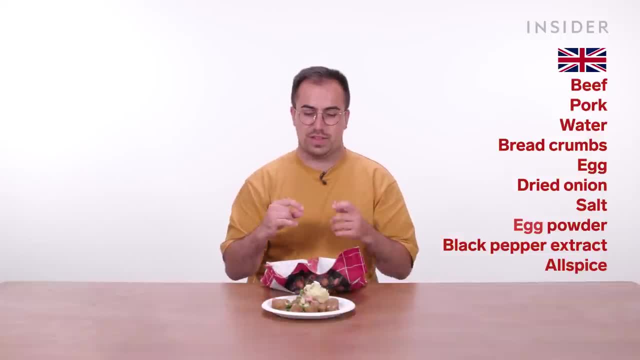 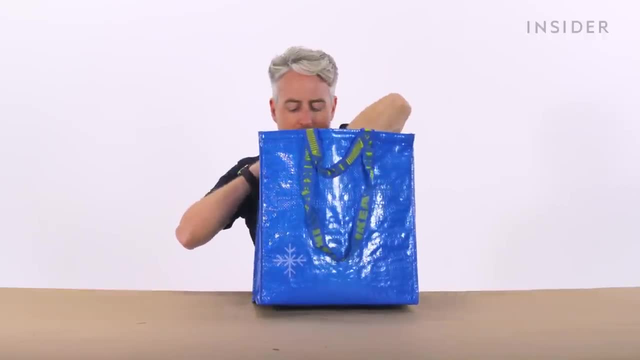 Overall, it seems like it's pretty close to the list that they gave you on the website, with a few more things like powdered ingredients versus fresh ingredients and a couple of spice differences too. I wasn't able to find it online or in the cafeteria. 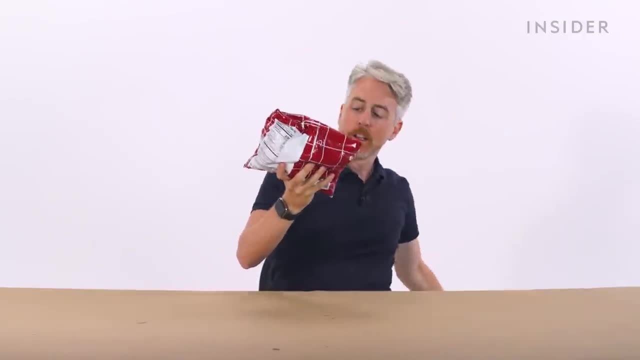 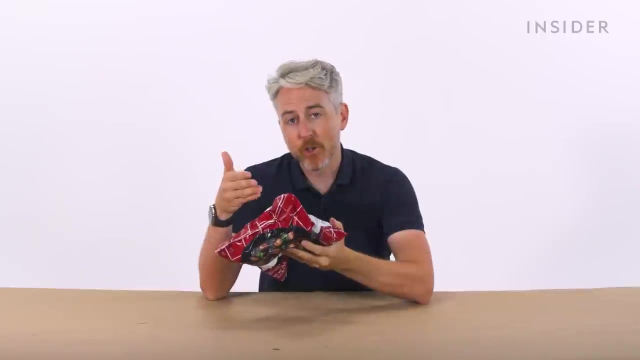 the ingredients list, but I got here the frozen precooked meatballs and those ingredients. Hmm, actually not bad, assuming these are the ones that they have in the cafeteria in the US. The ingredients for this is beef, pork, water. 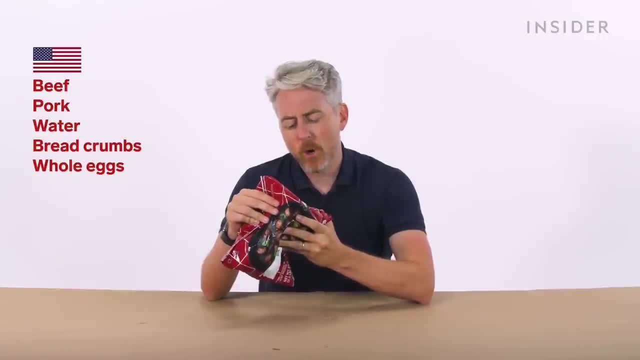 bread crumbs made of unbleached wheat, flour, salt, yeast, whole eggs, salt, dehydrated onion- a white, that's not plural, a white singular. spices, That's not bad, I think, for a prepackaged product right. 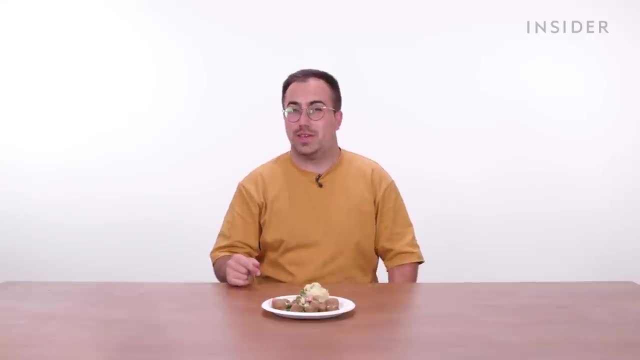 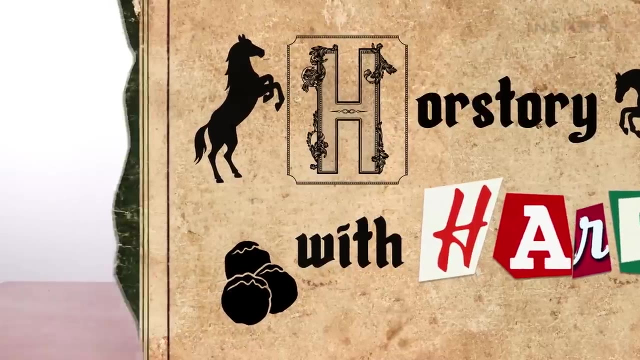 It's like you know. it's what's in them, right? While we're on the subject of IKEA ingredients, one thing that UK viewers might remember was our infamous horse meat scandal Back in 2013,. a number of foods in the UK claiming to be beef or pork. 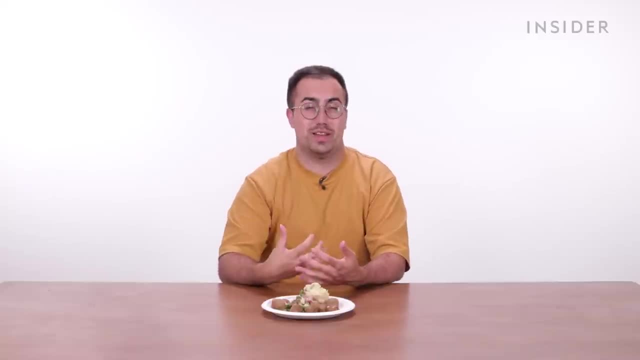 were actually found to contain traces of horse meat. While this wasn't necessarily a health issue, it did raise some major questions concerning the traceability of foods throughout supply chains, And unfortunately, IKEA was also caught up in this scandal. Czech authorities found traces of horse meat. 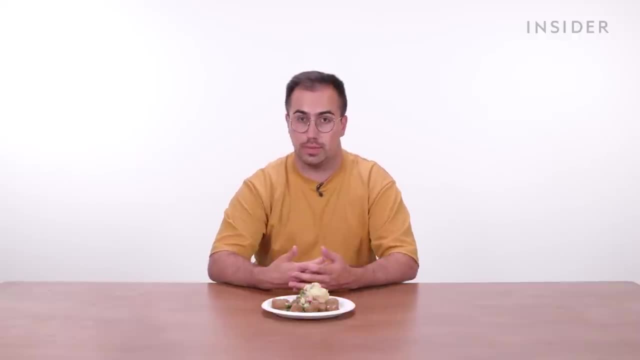 in some IKEA meatballs that had been produced in Sweden and shipped all around Europe. Thankfully, the horse meat meatballs were found before they reached consumers. In total, 760 kilograms of meatballs were destroyed. Given the fact that there's no health concerns, 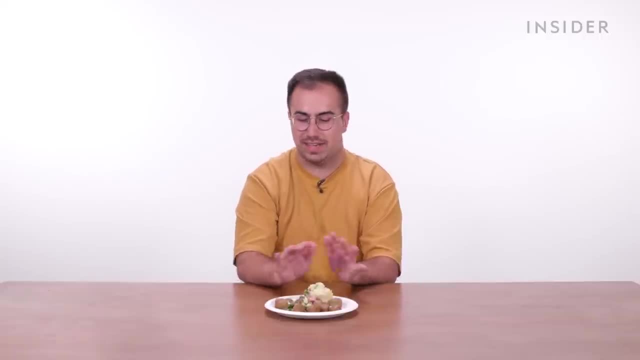 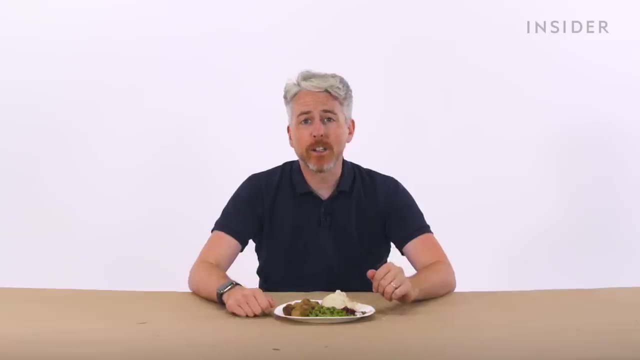 related to the consumption of horse meat. I think we should have just leaned into it. Just pass them off as like limited edition horse meatballs and just go with it. lads, It's fine. IKEA's food is almost suspiciously cheap. 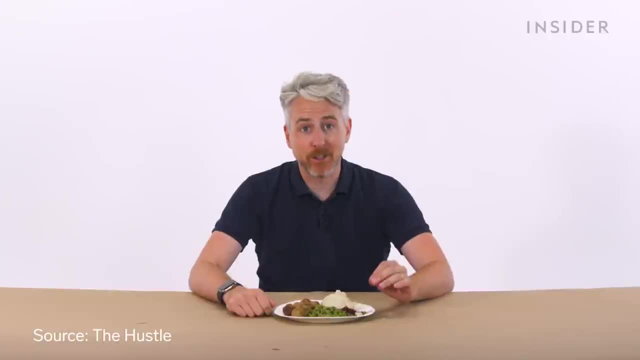 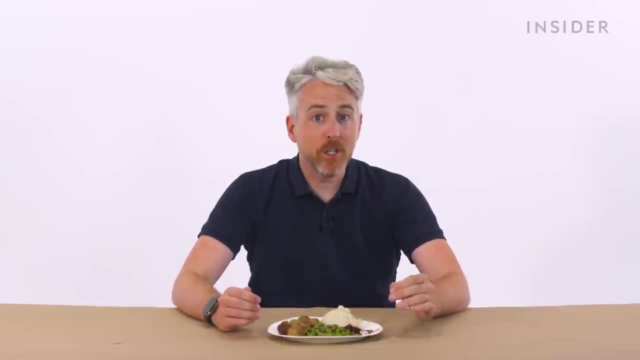 And it's actually one of the ways it tricks you into spending more time and money in its stores. IKEA is basically willing to take its losses with its cheap food prices because it's counting on you to spend a bunch of money on furniture and other household items. 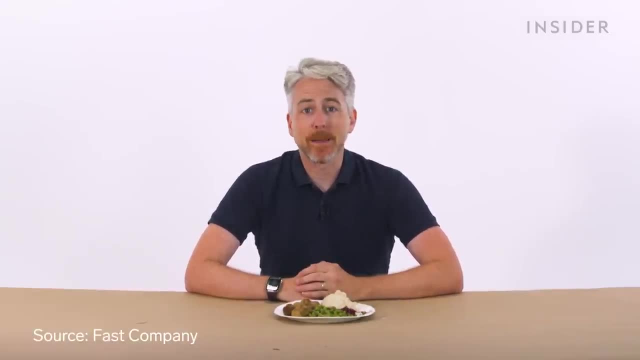 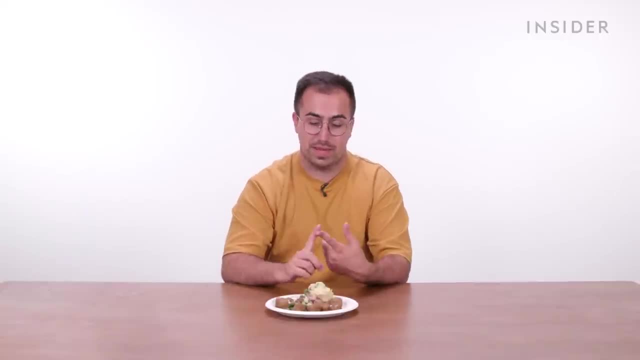 A former IKEA executive even referred to the meatballs as the best food. A former IKEA executive even referred to the meatballs as the best food. Sofa cellar In the UK a plate of eight meatballs, peas, mash or chips. 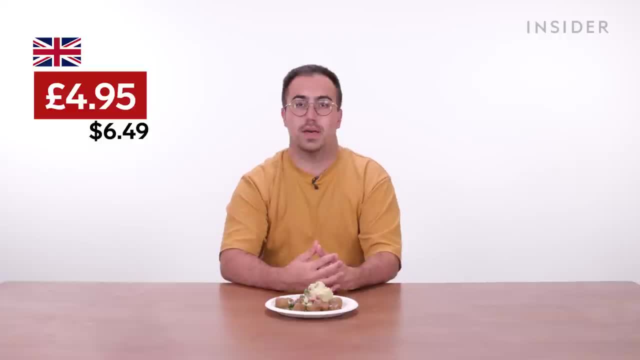 gravy and lingonberry jam will set you back just £4.95.. At the time of recording, that's around $6.49.. At the time of recording, that's around $6.49.. I do have to say that's really cheap. 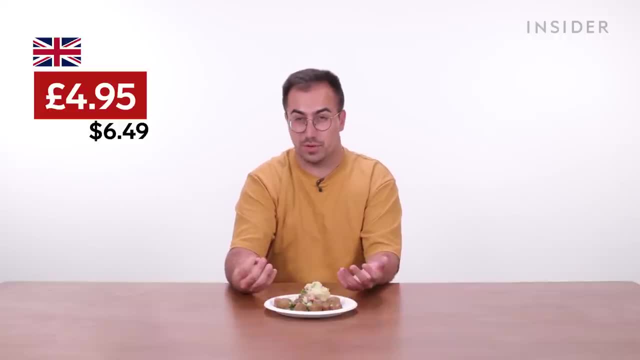 But I don't think the quality is that bad. It's really tasty food And yeah, it's a real bargain. I will make an effort to go via the restaurant if I'm just going for IKEA, Even if I'm just popping in for like one or two bits. 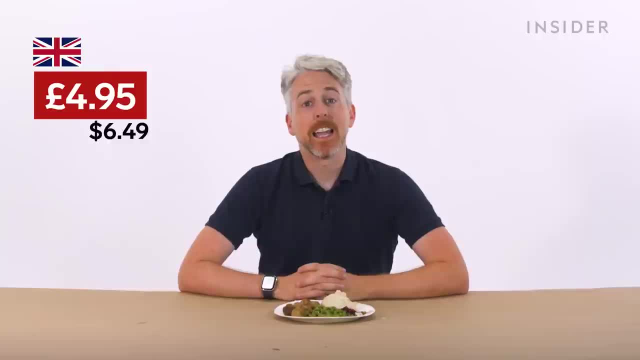 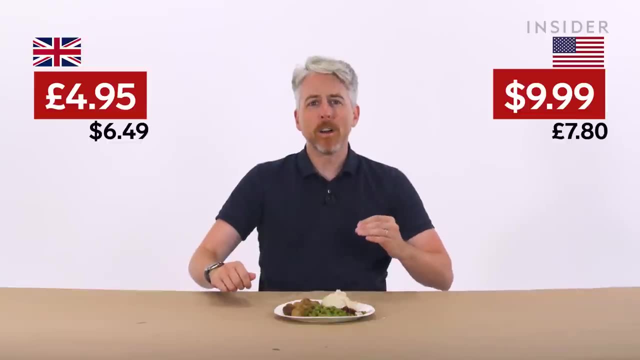 I'm gonna sit down eat a plate of meatballs. It's good value, It's tasty. eight meatball meal in the US is $9.99, which in the UK is £7.80.. That's a 54% increase in the. 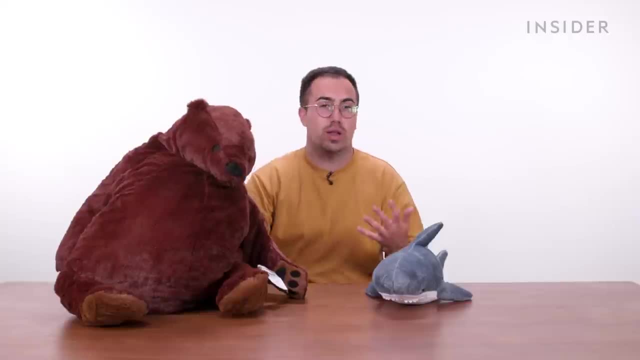 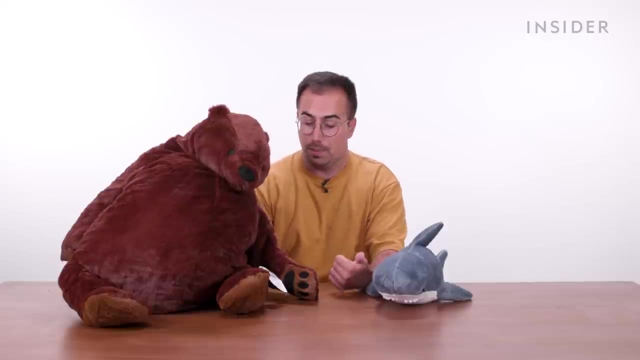 States. Overall, I would say Ikea is pretty popular in the UK. It's most people's go-to for basic furniture and household needs, I would say, especially when people are buying a house or moving house or something like that. Personally I love Ikea, I love going there. I do enjoy a trip. 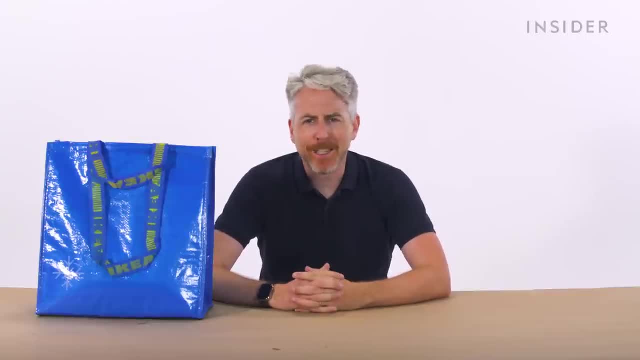 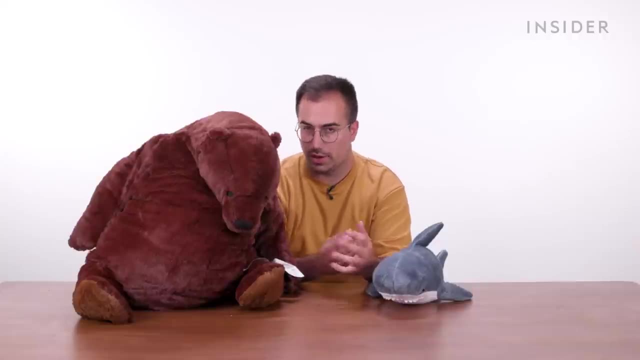 It's fun, I like the food, I like walking around and pretending like, ooh, that could be my apartment or my bedroom or my kitchen. I wouldn't say. Ikea is somewhere I go often, particularly because I live in quite central London and there aren't many in central London. I think they're. 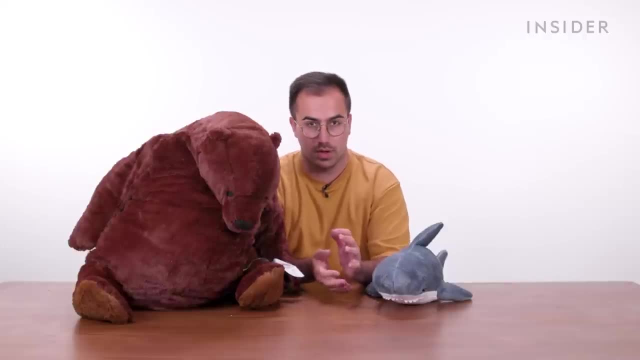 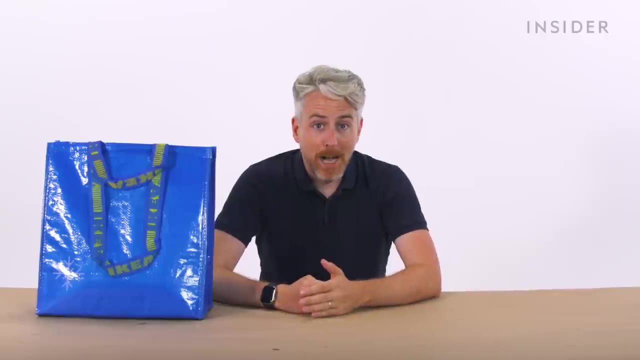 trying to open one on Oxford Street right now. At the time of recording this it wasn't open, but they're kind of trying to get there. But so, like I say, it's more of a place where you'll go specifically when you need to do an Ikea shop. Ikea is so popular here, I think it's popular. 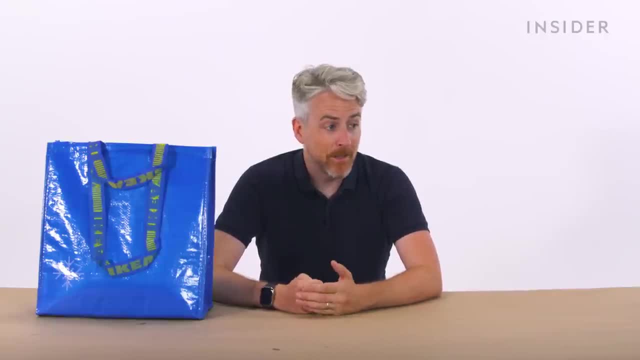 in the whole country, The one in Burbank. we went there at 10.30 in the morning. It opens at 10, and at 10.30, the parking lot was pretty full. The cafeteria line was full, So I'd say Ikea is. 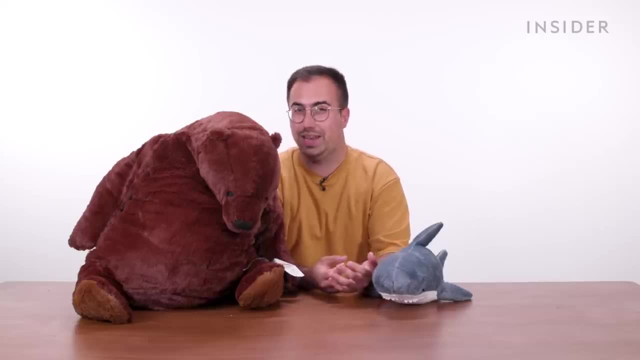 pretty popular. I personally wouldn't go to Ikea just for the food. Again, it might be because I don't live close enough to one to make that worthwhile. I do love the food. The meatballs are great. Like I say, the desserts are fantastic, but I don't like it to the extent that I would. 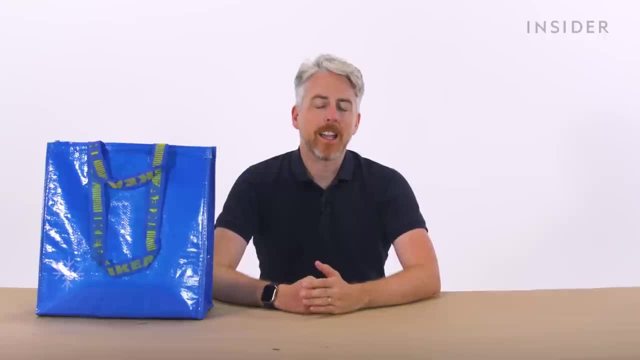 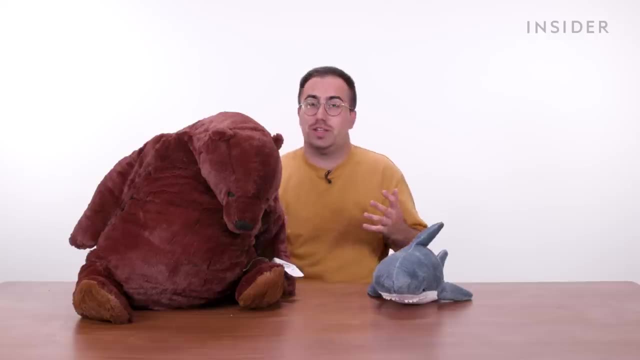 make the effort to travel to one just to eat there. I'm not going to say I go to Ikea for the food, but the food definitely is a good motivator to go to Ikea. I will say overall I do enjoy the experience of going to an Ikea. I am aware that it's kind of designed to make us spend money. 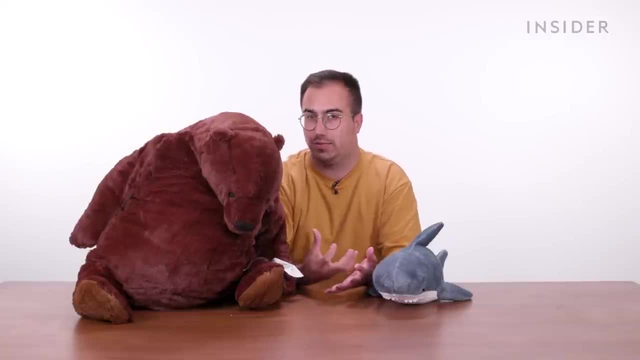 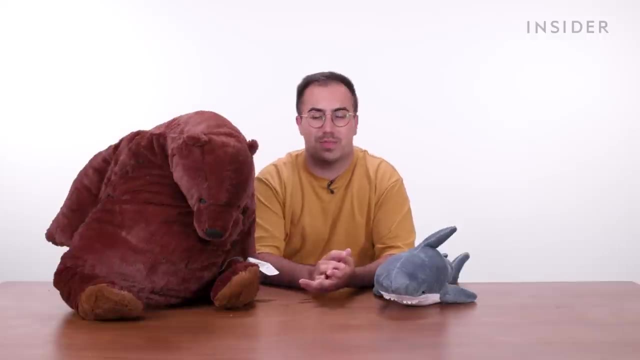 Obviously, the restaurant plays a part of this as well, because it's kind of encouraging you to make a day of your trip to Ikea. Really spend some time there, Sit down, take a break in the middle of the day, eat, re-energize yourself for more shopping And, as you can guess, by my friends on the table, 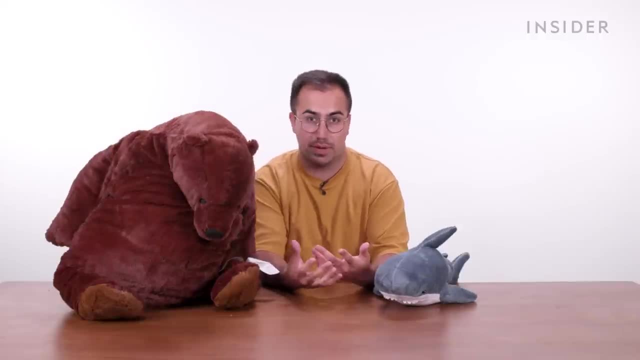 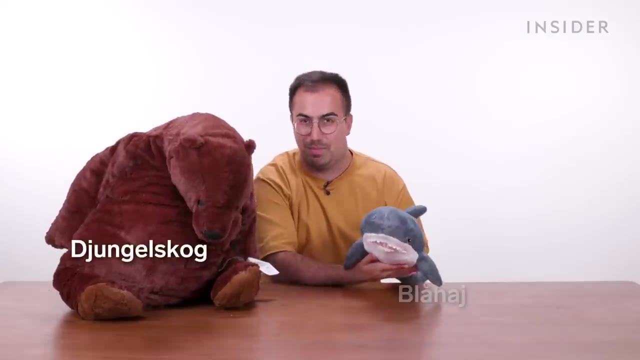 with me here. I do think that their marketing is a really clever ploy to make us spend more money there as well. I'm joined here by my friend Dungl Skog- I'm really sorry I'm going to butcher these pronunciations- And my friend Blahai, who is the adorable little shark who is also 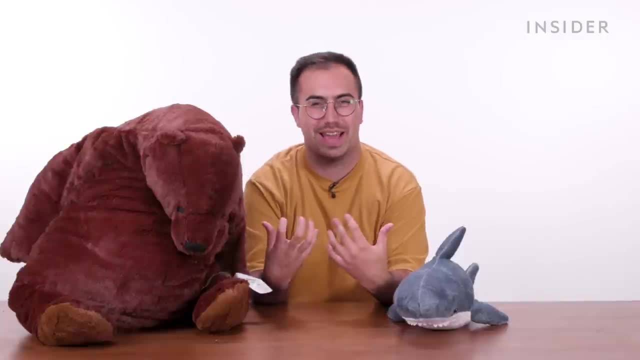 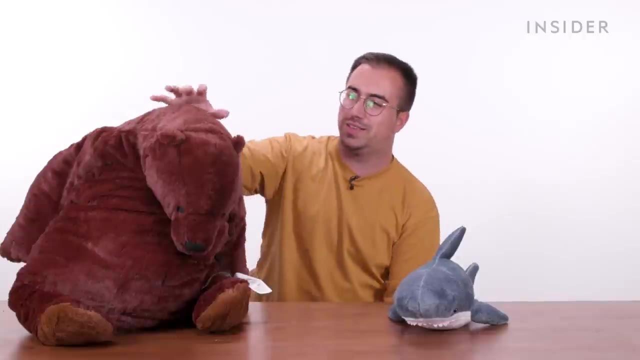 I think a trans icon Love that You'll often see things like this really getting like a reputation on the internet, driving more commerce to Ikea stores. I don't know if they're doing that deliberately or if it's just kind of like a side effect of making some very, very cute plush. 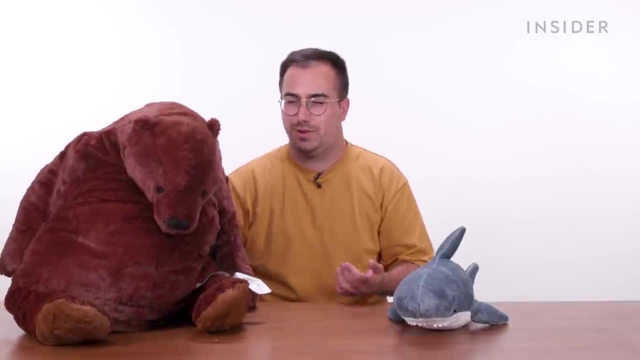 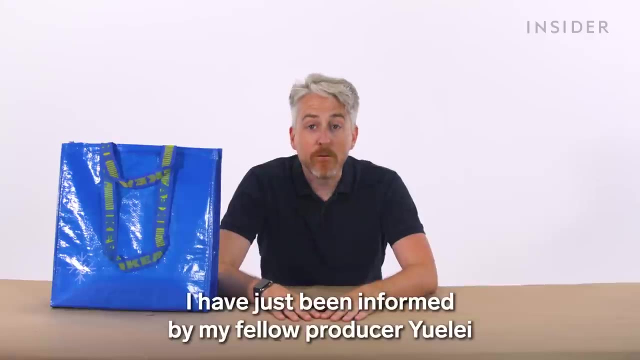 toys, But everyone, I think, will generally have at least one thing from Ikea in their home. So whatever they're doing, it's kind of working. I'm not mad about it either. I support Ikea. Keep up the good work, guys. I've just been informed by my fellow producer. 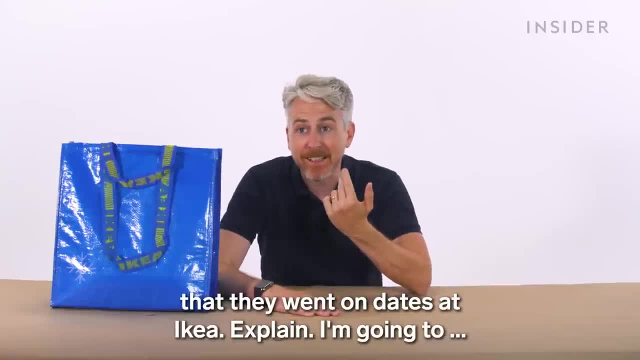 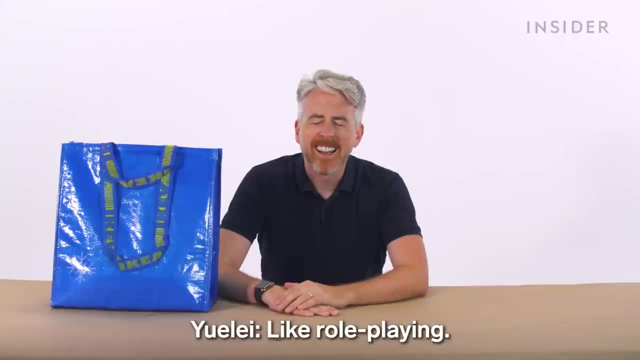 Yuli that they went on dates at Ikea. Explain I'm going to They kind of do pop-up a couple. It's like something you can do. Yeah, I didn't think That's a good way to get to know someone. First you start eating. 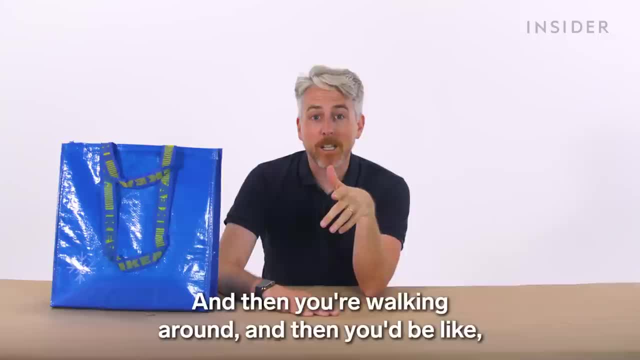 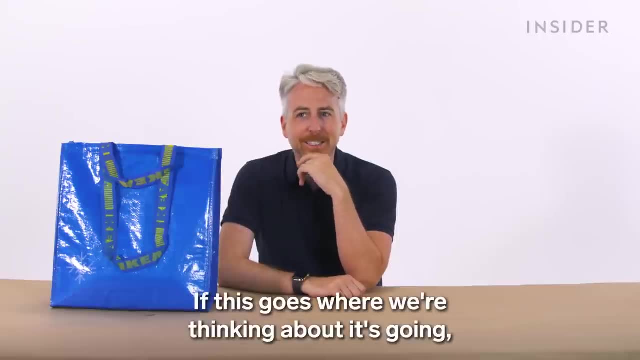 The food's dirt cheap, so Great, Okay, great. And then you walk around and they'd be like: this is the kind of couch I like, It's the kind of art I like, And you're like: no, they're into that. huh, If this goes, we're thinking about it going. this is the kind of. 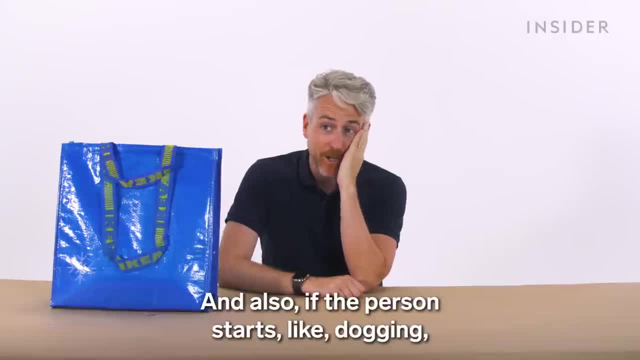 bedroom set if they want them, I don't know. And also if the person starts like dogging- like you see something that you like and they start dogging on it, you're going to be like this isn't going to work out. This isn't going to work out. What kind of weirdo wants a closet? 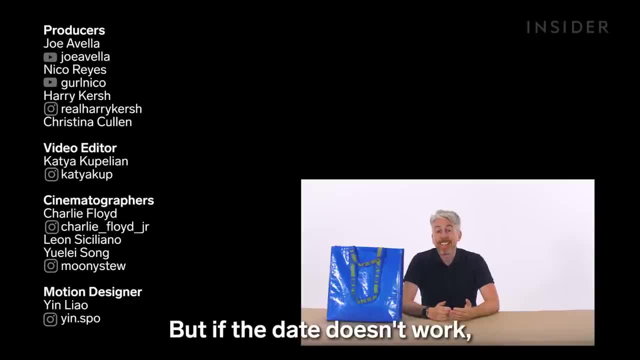 like this: You're like: I do Take me home, But if the date doesn't work, that's like a long walk out of there. Silence, Yeah, And if you get to the kids area it's all like the kid stuff and 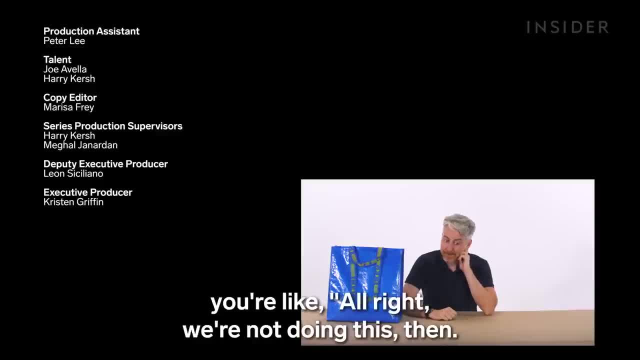 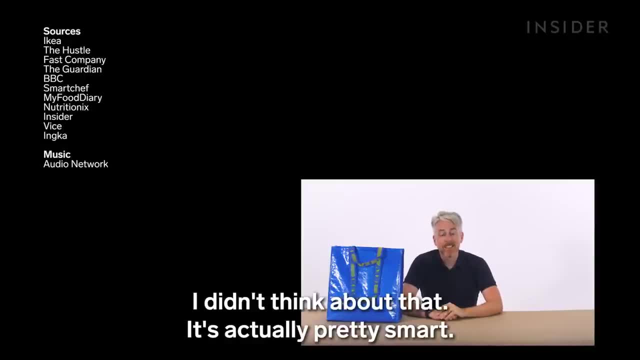 the baby stuff And if your partner's like I don't want any of this crap, you're like, all right, we're not doing this, Keep walking That actually. Yeah, it's actually a good idea. Yeah, All right, A date at Ikea? I didn't think about that. It's actually pretty small. All right. 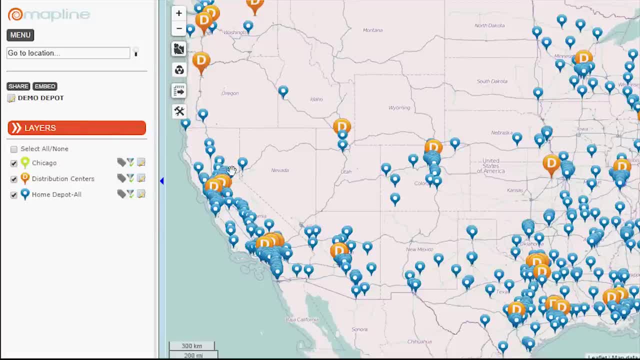 This video is about distance calculators. If I wanted to figure out the distances between two of my datasets, so the distance from my retail stores to my distribution centers or the distance from my distribution centers to the city of Chicago, I can use this button here.